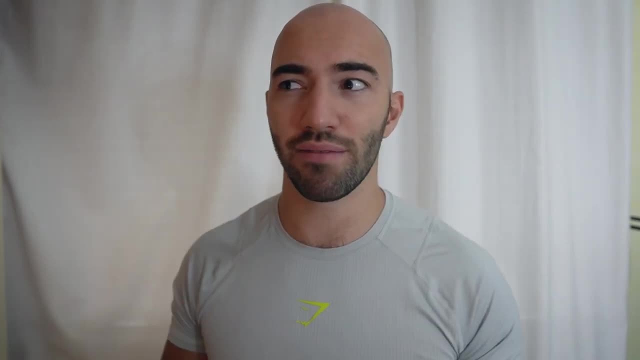 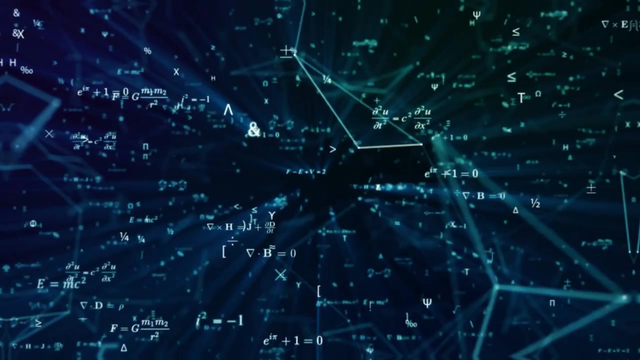 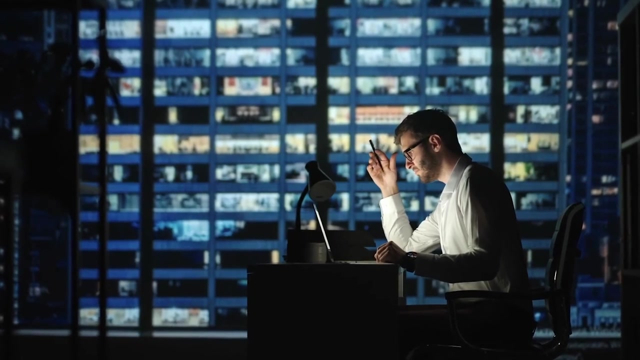 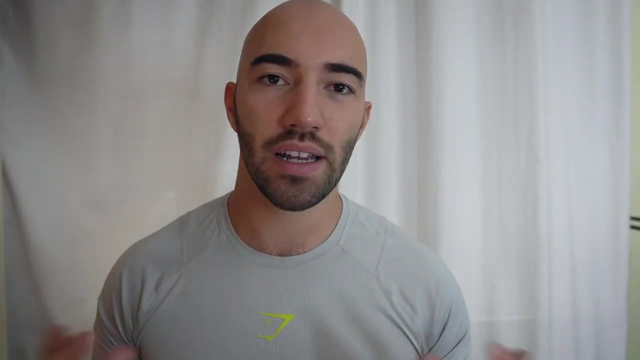 convolutional networks had been around for a while, but using them had kind of been deemed impractical. yet when AlexNet's results came in it proved sort of unparalleled performance on what was seen as the one of the hardest challenges of the time. So this event made AlexNet the first widely acknowledged successful implementation of deep 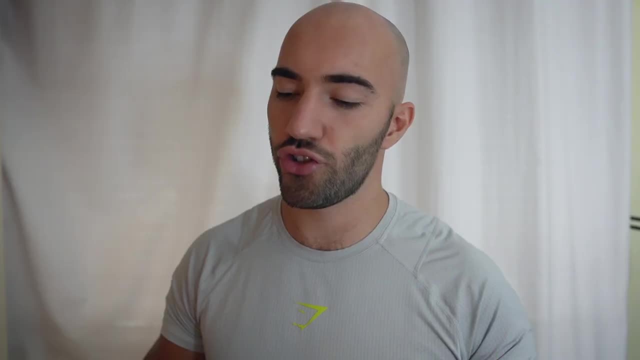 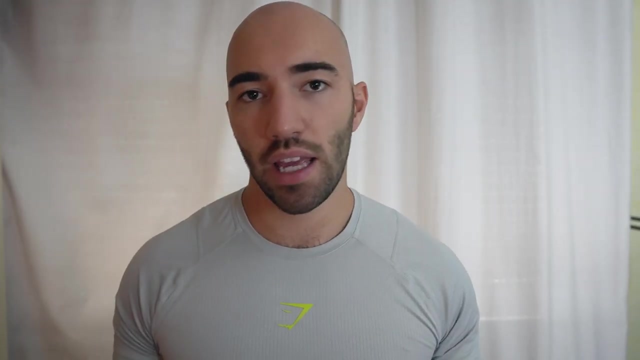 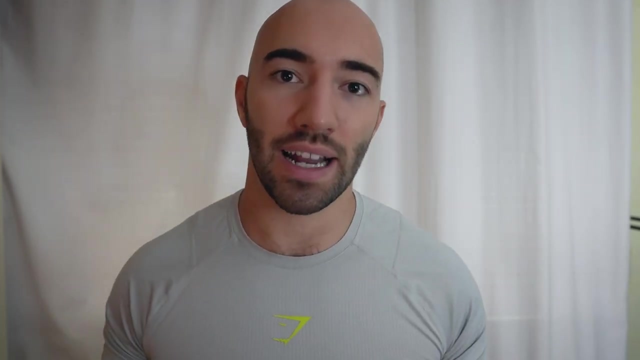 learning and the sheer performance improvement that it showed caught people's attention. Until this point, deep learning was unproven. It was simply a nice idea that most people just decided: okay, it's impractical, we don't have enough data, we don't have enough compute to. 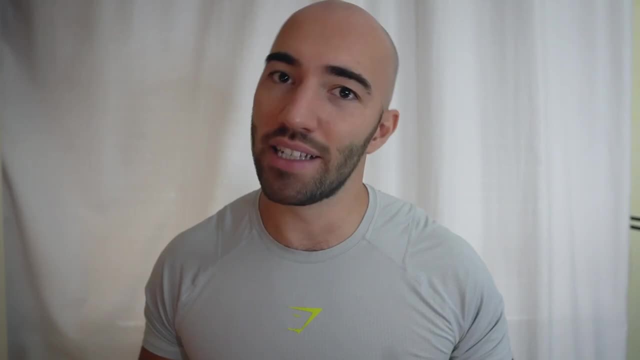 to do anything like this. But AlexNet showed that this was not the case and that deep learning was now practical. Yet this surge of interest in deep learning was not solely, you know, thanks to AlexNet. ImageNet also played a big part in this, The foundation of applied deep learning. 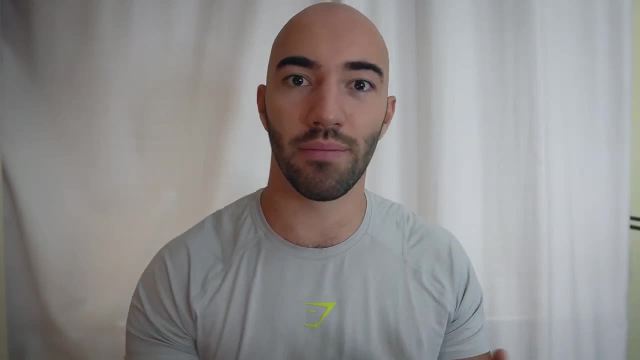 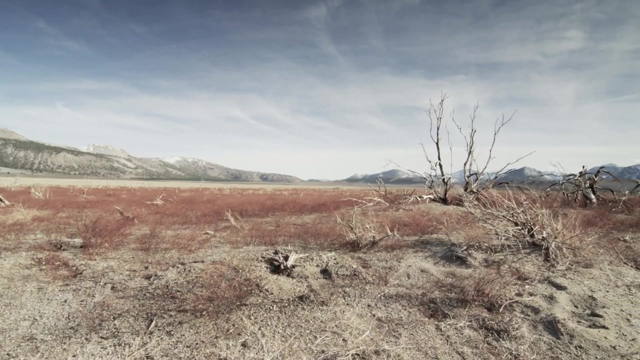 was set by ImageNet and built upon by by AlexNet. So let's begin with ImageNet. Back in 2006, the world of computer vision was a lot different to how we know it now. It was pretty underfunded. It didn't really get that much attention. Yet there were a lot of researchers. 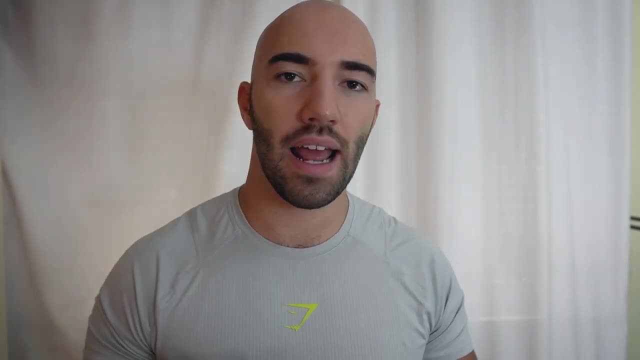 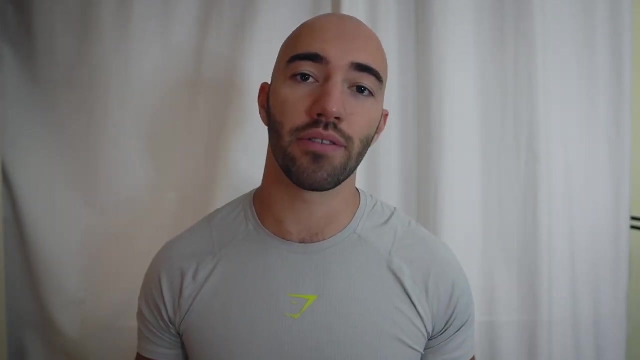 around the world focused on building better models, and the year after year they saw progress, but it was slow. In that same year, a woman called Fei-Fei Li had just finished her computer vision project and had started working as a professor in computer science and had noticed this sort of 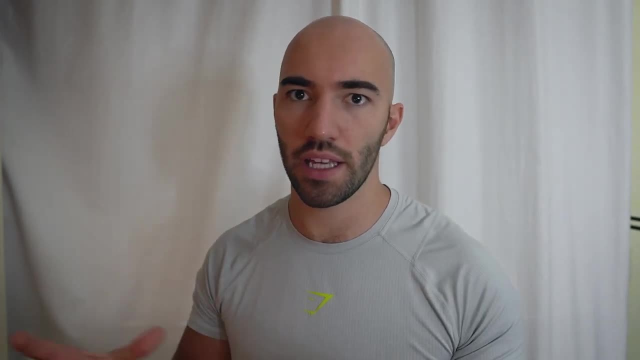 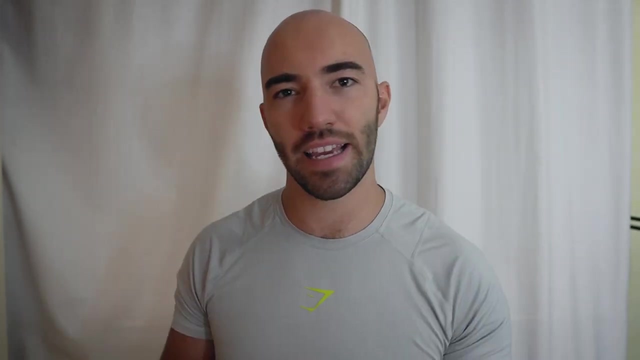 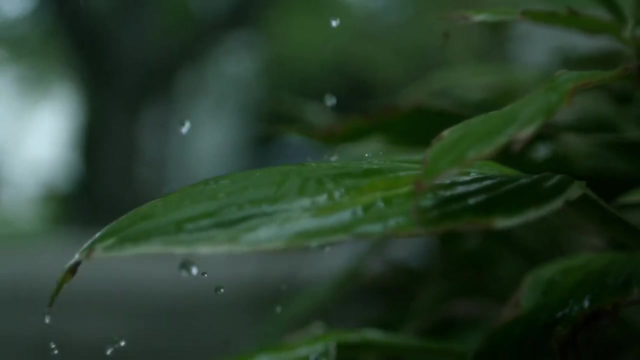 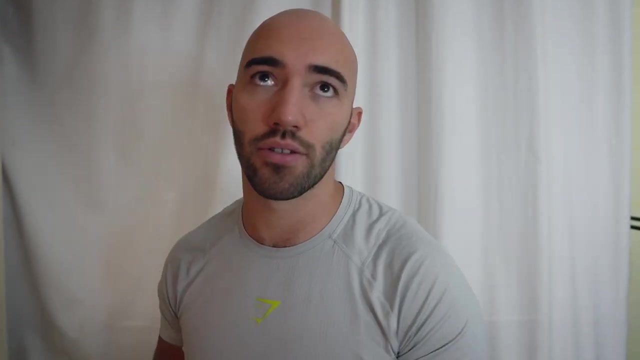 focus in the field of computer vision on the models and the subsequent lack of focus on data, And an idea came to the that maybe a data set that was more representative of the world could improve the performance of the modelers being trained on it. Around the same time as this, there was another professor called Christiana Felbom and she was a. 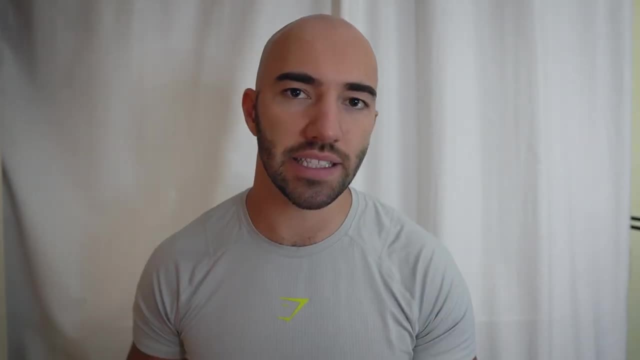 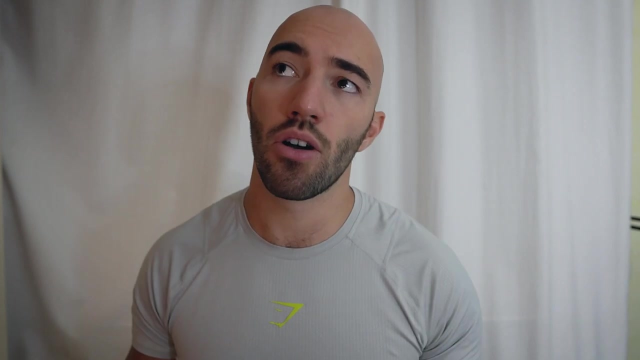 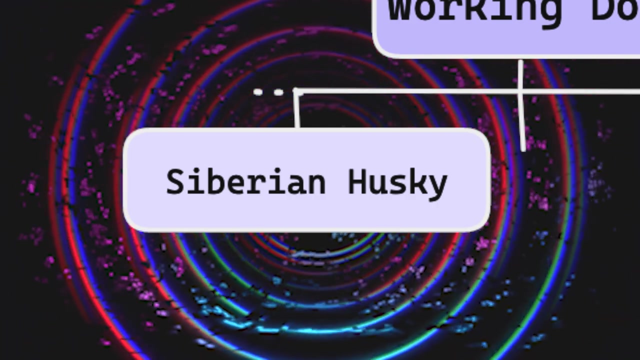 co-developer of a data set from the 1980s called WordNet. Now, WordNet consisted of a pretty large number of English language terms organized into an ontological structure. So for example, for the term Siberian Husky, that would be within a tree structure and above Siberian Husky, you would have 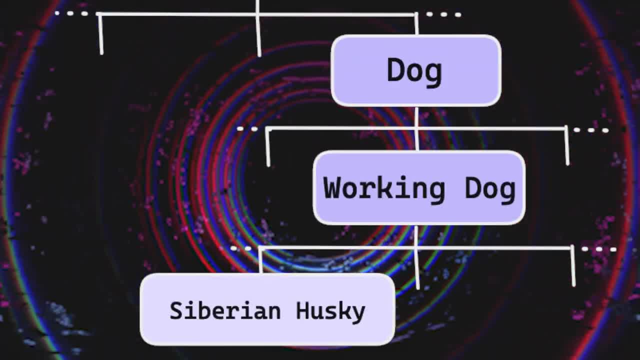 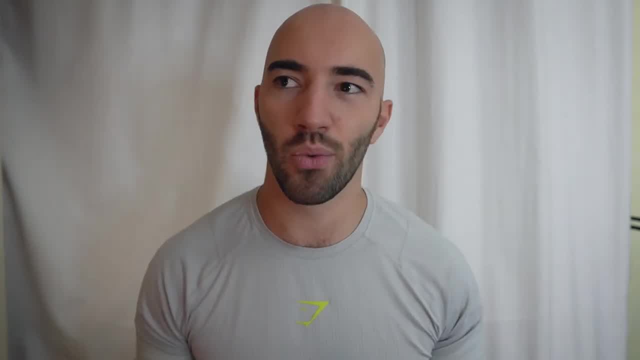 working dog, Above working dog, you would have working dog, and above working dog, you would have working dog, You would have dog above dog, you'd have canine carnivore and so on. So there's like that tree structure of different terms and where they and how they relate to each other. In 2007, Li and 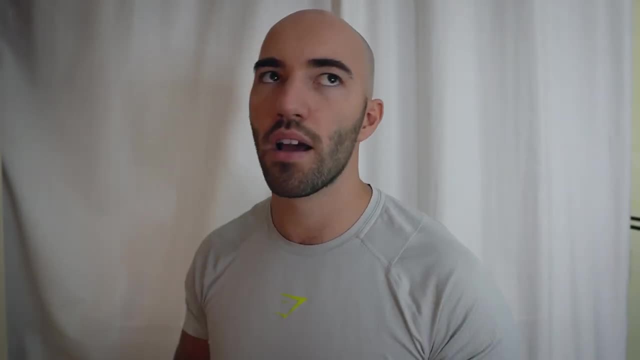 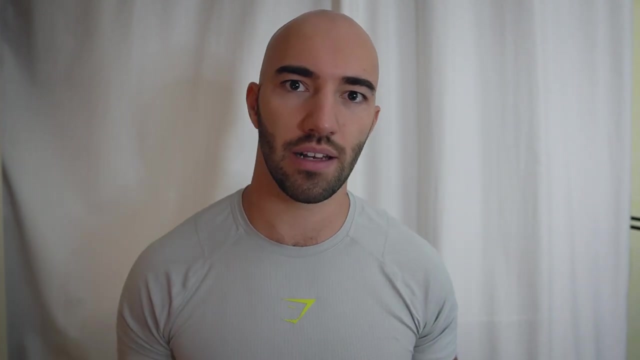 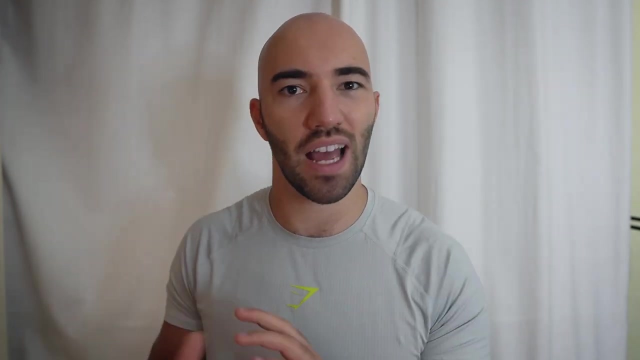 Felbom met and Felbom discussed her work on, or her idea at the time of adding just a reference image to each of the terms within WordNet. So the intention was not to create a image data set, but it was simply to add like a reference image so people could more easily understand what that particular 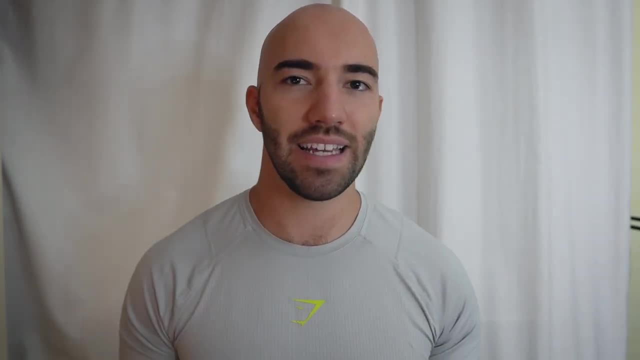 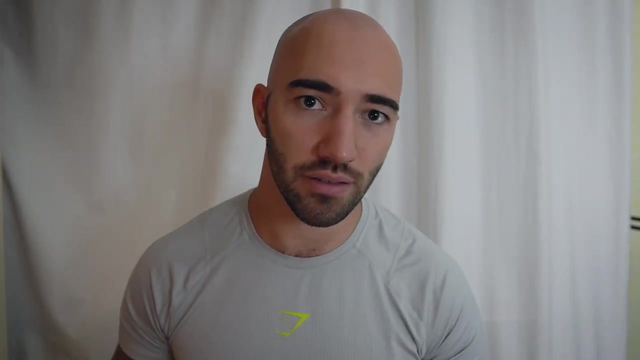 term was about, And this inspired an idea from Li that would kick-start the world of computer vision and deep learning. So soon after, Li put together a team to build what would become the largest labeled data set of images in the world, called ImageNet. The idea behind ImageNet was that a large 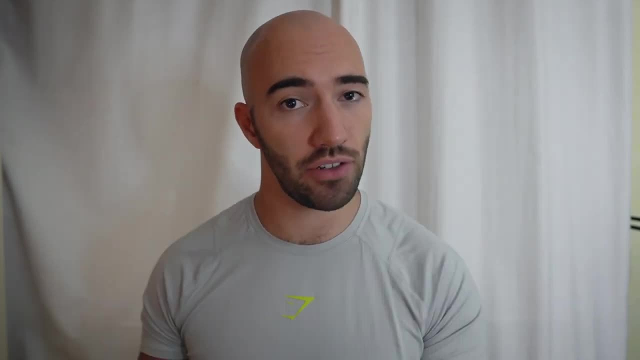 based data set like WordNet, but for images, could be the key behind building more advanced content based image retrieval, object recognition, scene recognition and better visual understanding in computer vision models. And just two years later, the first version of ImageNet was released with 12 million labeled images. These were all structured and labeled in line with the 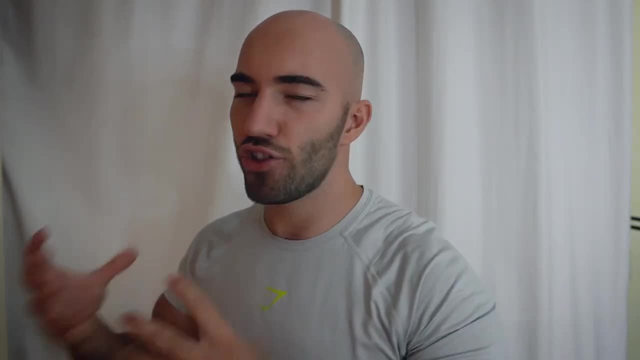 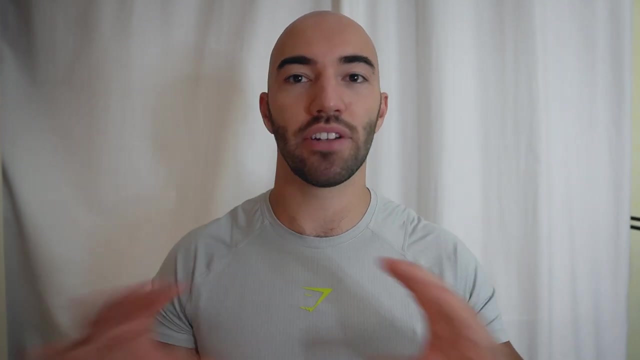 WordNet ontology. Yet if we consider the, the sheer size of that, the the 12 million images, if one person had spent literally every single day labeling one image per minute and did literally nothing else in in that time- they didn't eat, they didn't sleep, just just labeled images- it would. 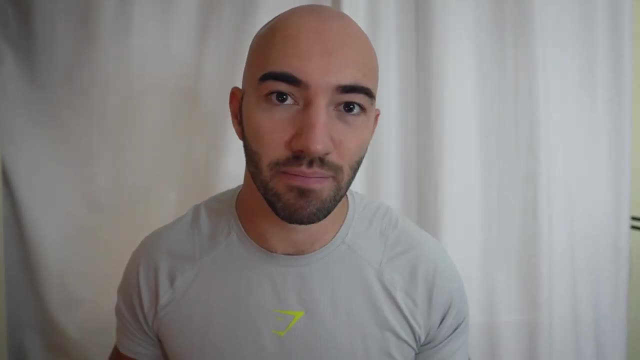 have taken them 22 years and 10 months, Which obviously is a very long time. There's just an insane number of images to be labeled here. So how? how did they do it? Because the team was not huge, they didn't have like an infinite amount of money to pay other researchers and students to do this. 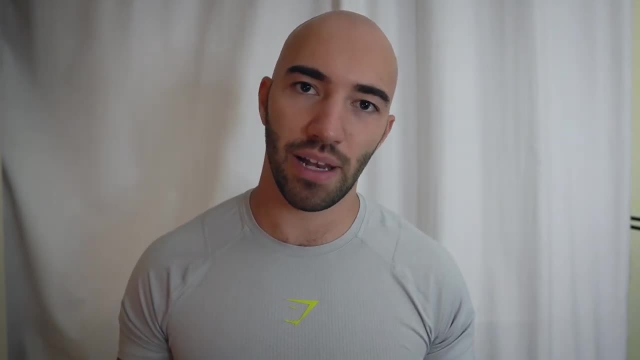 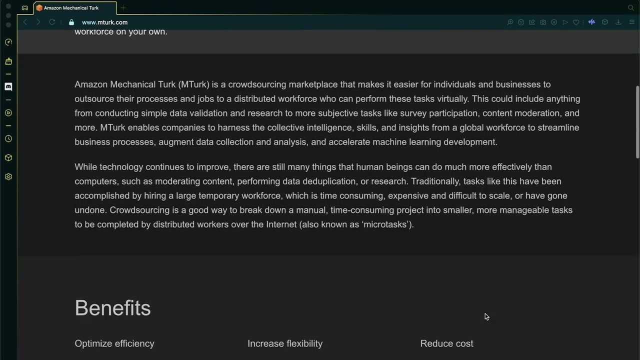 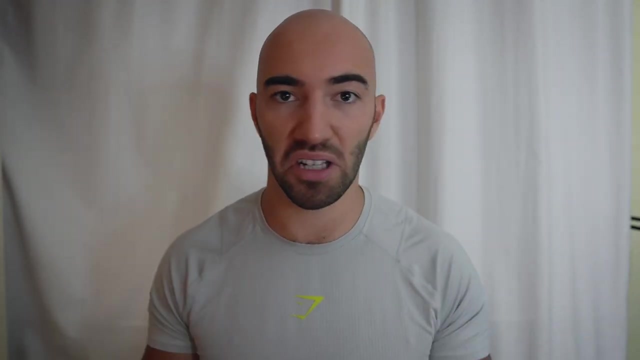 So what they eventually settled on was a platform called Amazon's Mechanical Turk. Mechanical Turk is a crowdsourcing platform where people from around the globe will perform tasks such as labeling images for a set amount of money, And because there's just the insane scale of people around the 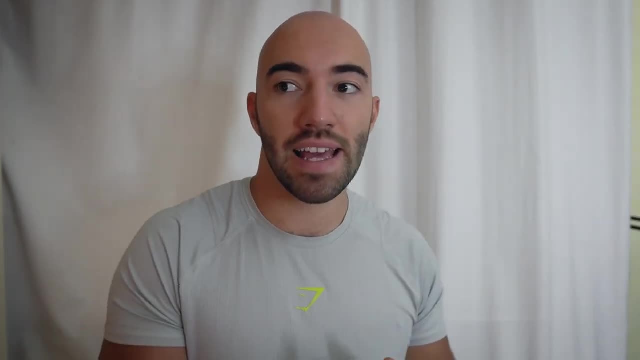 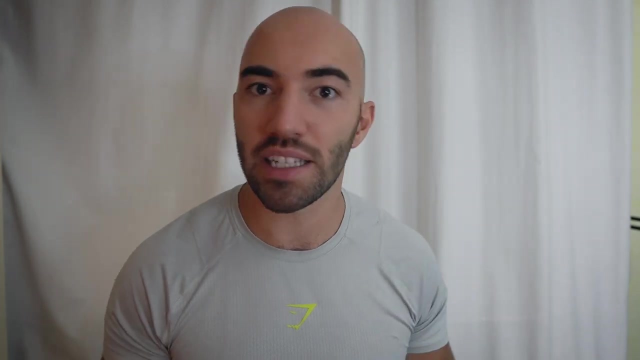 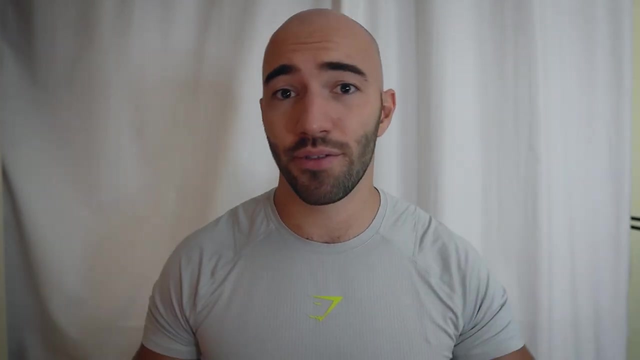 world doing this at competitive prices. that made ImageNet possible with a few adjustments to the labeling process, Because in reality, if you just have random people around the world labeling your, your data set, some of those people are going to try and take advantage of that, Maybe game the system. 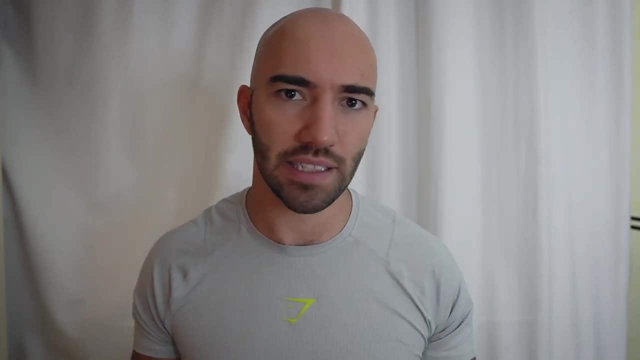 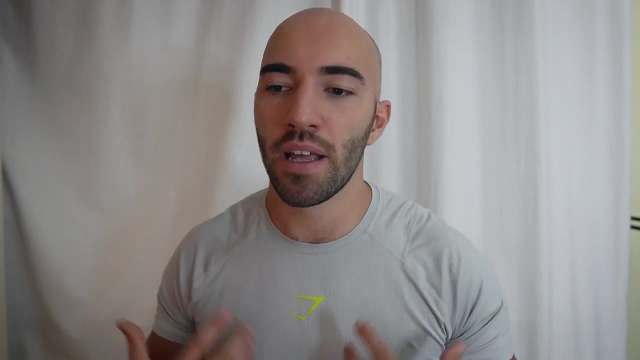 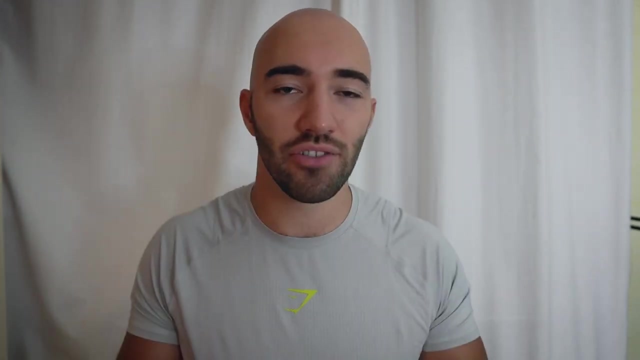 so you have to have some checks and balances in place against that. so you know there's a little bit of system design in there, but that is how they built the data set. now, on its release, ImageNet was the largest publicly available labeled data set of images in the world. yet 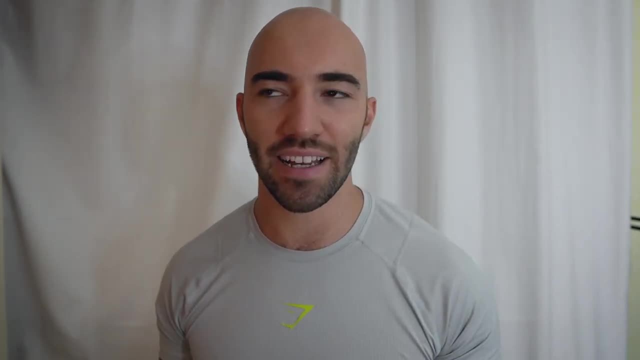 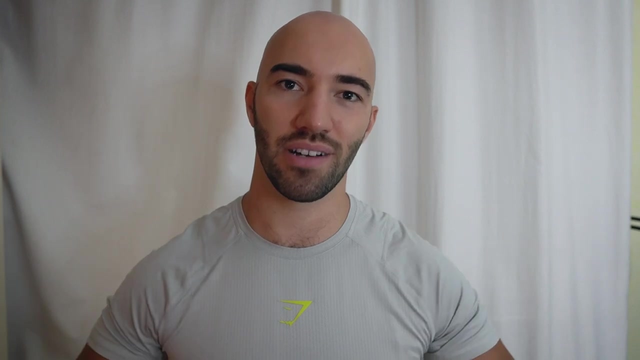 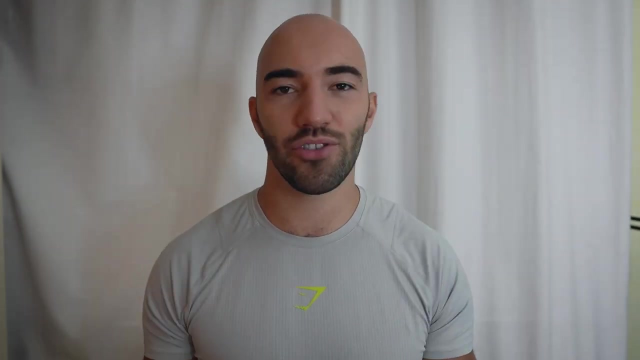 there was very little interest in the data set, which seems pretty crazy when we look back on that in hindsight, because now we know, okay, we, we want more data for our models to to make them better, but at the time things, things were different, so ImageNet came with these 12 million. 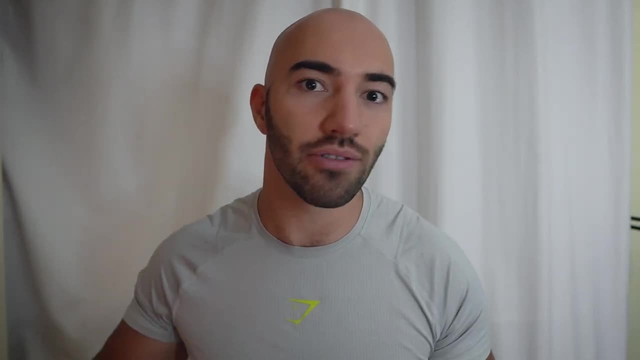 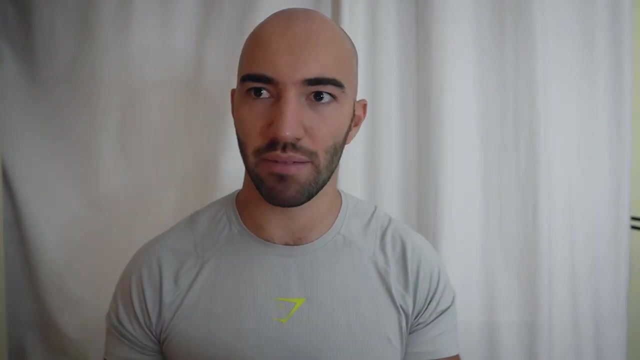 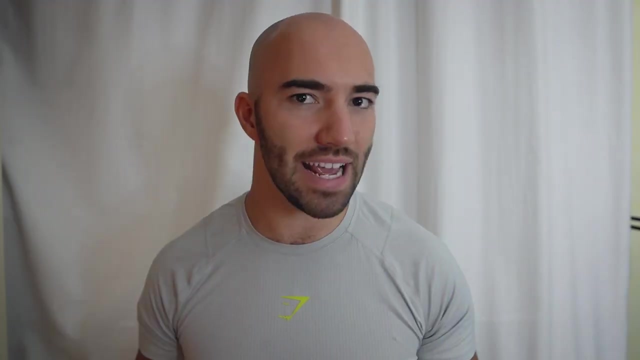 images distributed across 22,000 categories and at the time there were the odd other image data sets that used a similar sort of structure and idea. so, for example, the ESP dataset use like something called the ESP game and people would play the ESP game and label images for the for the dataset. now, reportedly, they 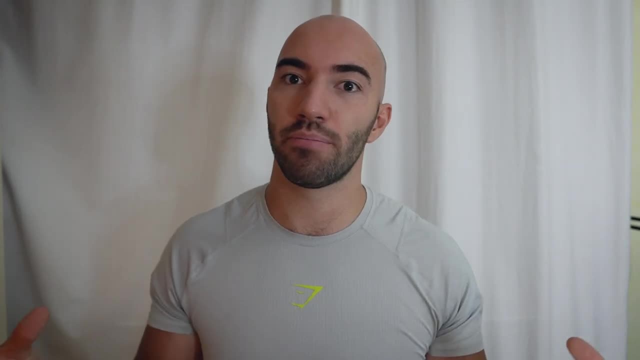 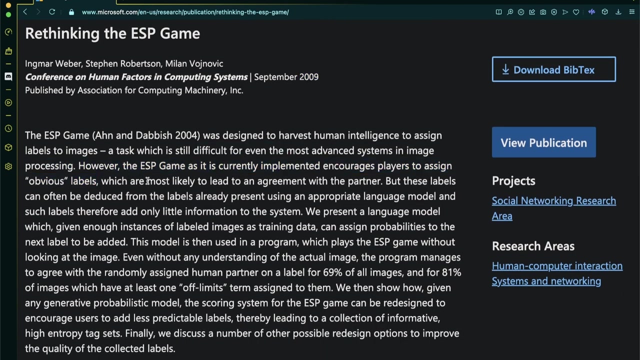 had way more images but it wasn't publicly released, only publicly released 60,000 of those of those images. and a couple of years later there were a few papers that kind of looked at the ESP game and ESP dataset and said, okay, it's probably not actually that useful because 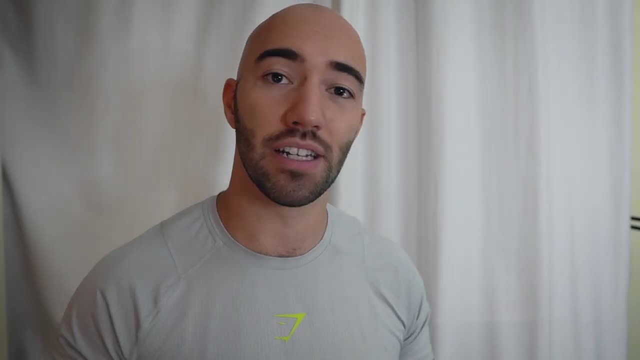 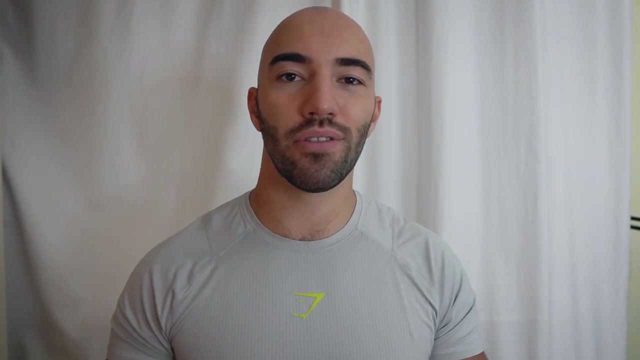 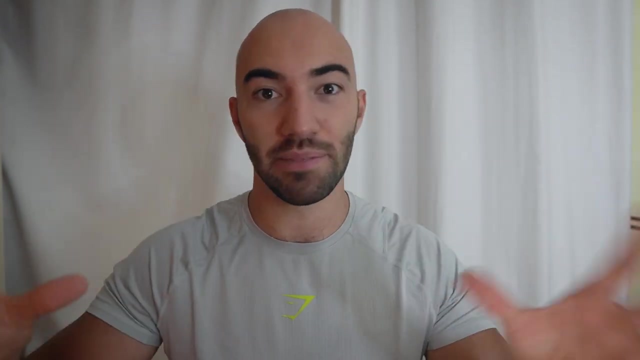 you can kind of guess the right answer most of the time without even looking at the image. so there were some questions around the usability of that dataset. so, all this to say, ImageNet was by far the the biggest, at least publicly available and and most sort of accurate. 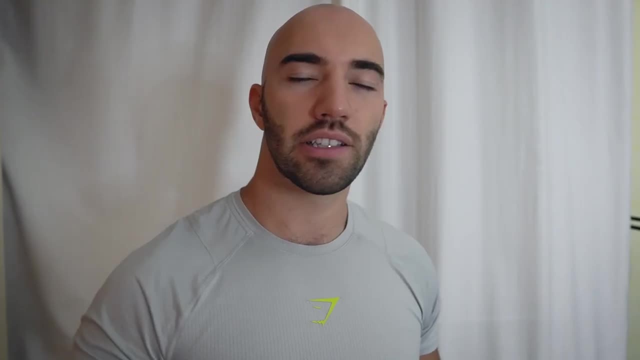 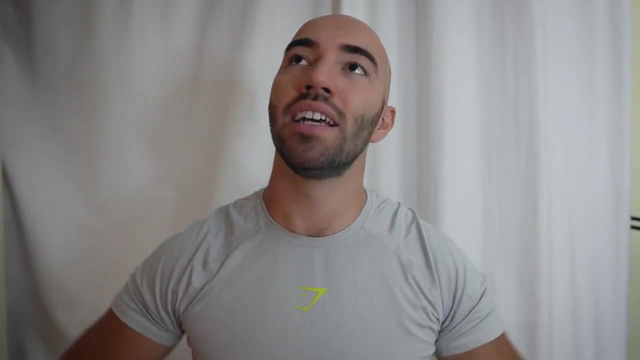 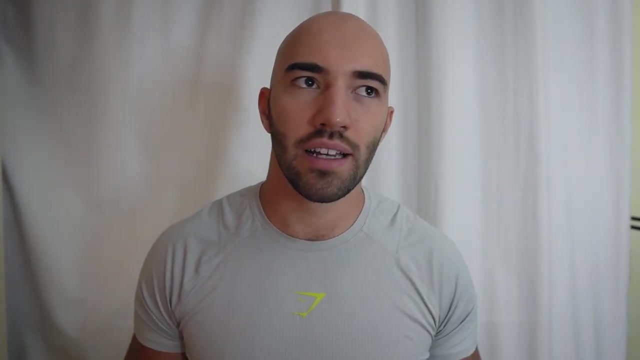 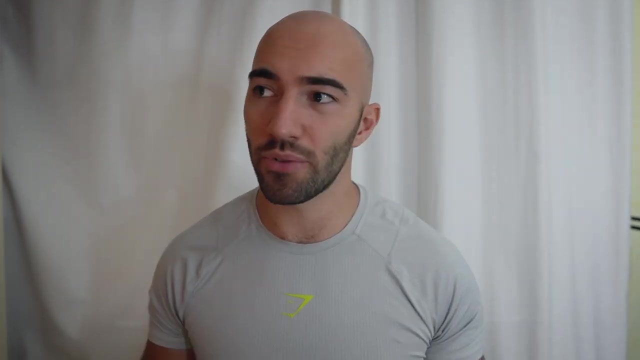 uh, dataset for computer vision at the time. so the reason that there was very little interest in ImageNet, despite its huge size, is that people just assumed that it could not work for their models. like you have to think back then they were training models on much smaller datasets which had 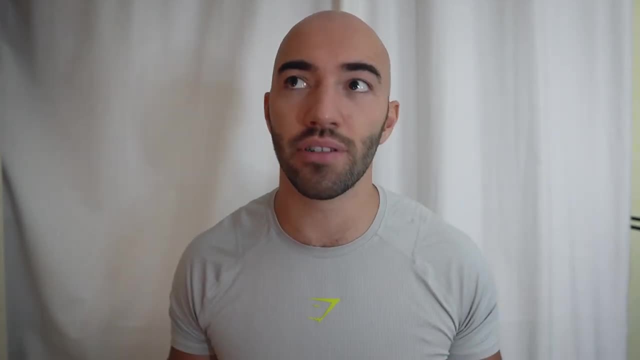 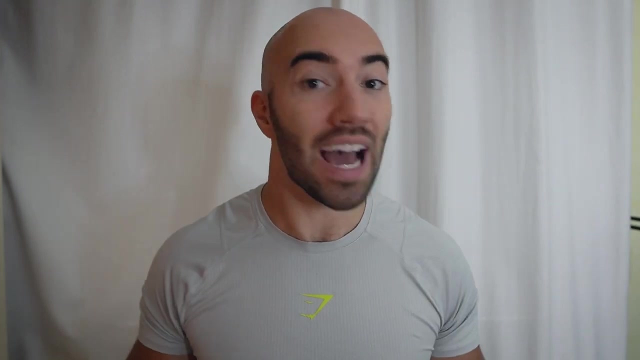 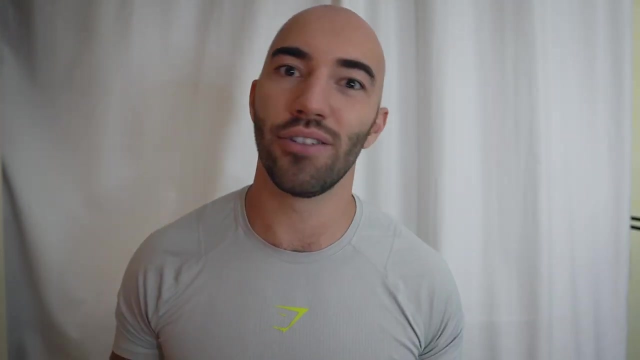 like 12 categories of images, for example, and the models would be more durable with that. so when ImageNet comes along and it's like, hey, I have 22,000 categories here, uh, people are just like, well, I can't deal with 12, so I'm not going to even try 22,000. that's crazy. 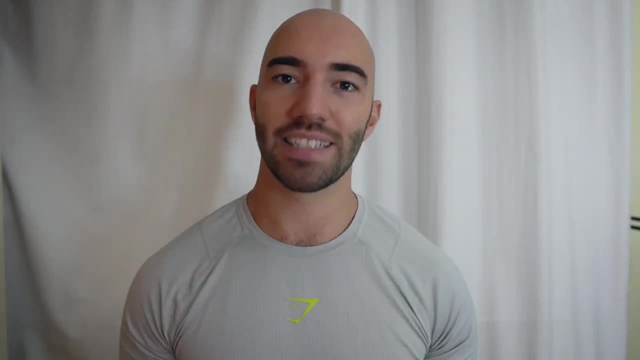 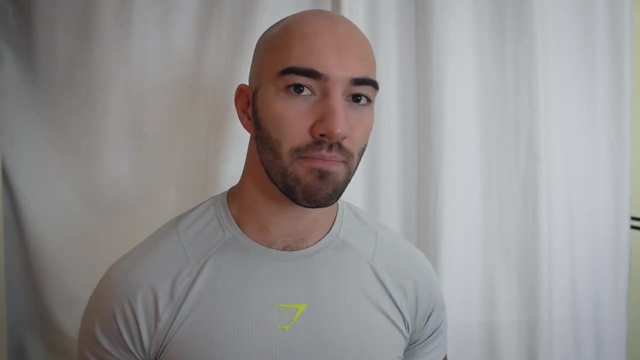 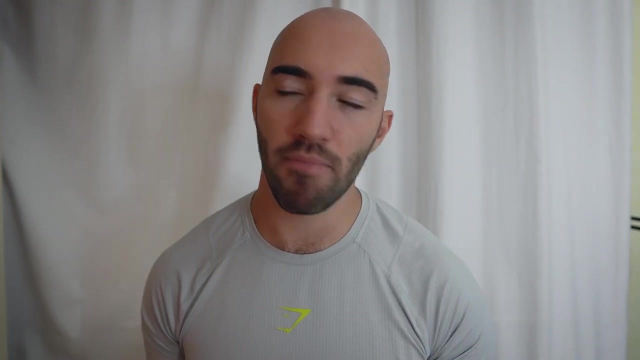 so there was a lack of interest in ImageNet at the time. um, it just wasn't really received that warmly. so the ImageNet team decided to, to you know, try and push it a bit more. so by the next year, 2000 and 10, they had managed to organize a, a challenge with the dataset, a classification challenge. 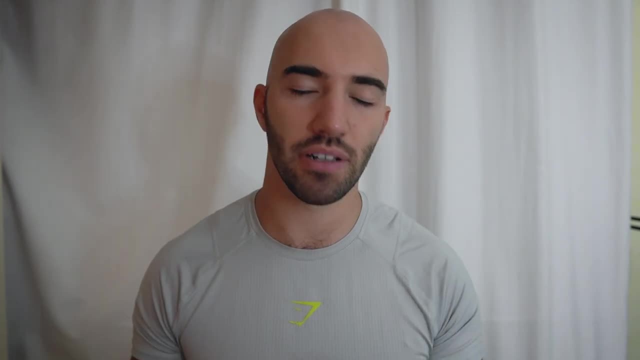 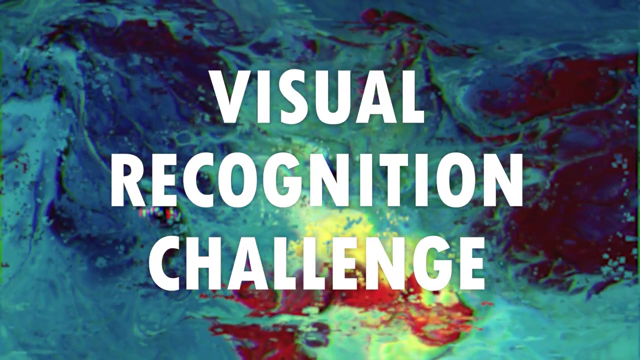 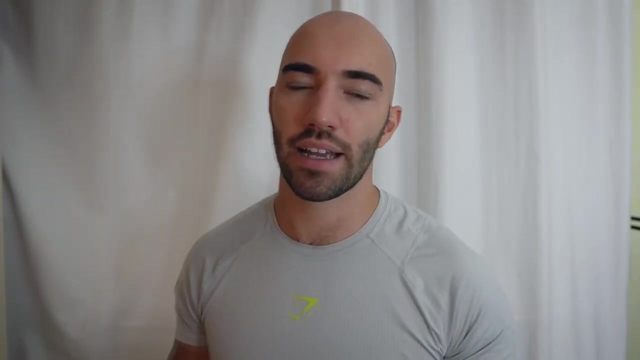 initially and they they grew into different things um over the years. but initially it's just a classification challenge. so the ImageNet large scale visual recognition challenge was first hosted in 2010 and competitors had to correctly classify images from 1,000 categories, so not just. 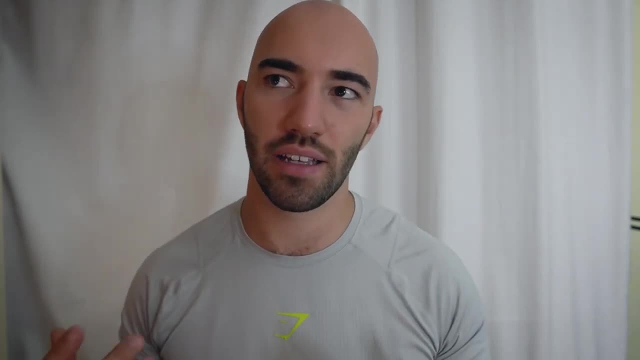 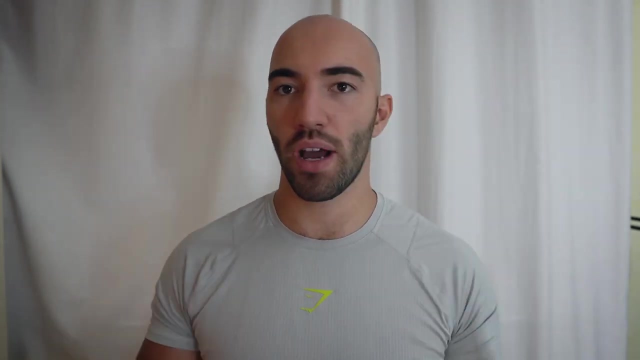 not a full set of terms in the in the ontology of ImageNet, but they had 1,000 categories in set and whoever produced the model with the lowest error rate won. okay, and and there were a few entrants, so there was not a huge number of. 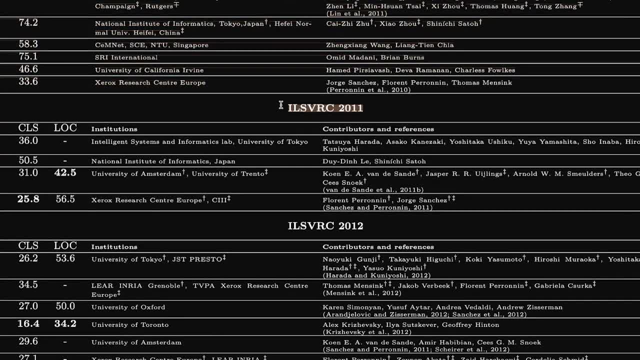 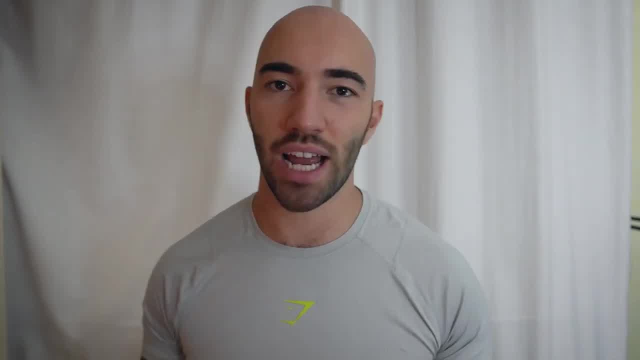 entrants. I think it's something like four or five, six entrants in the first, in 2010, 2011, 2012, now, eventually, this challenge will become the primary benchmark in computer vision progress, but it took some time and that really started in 2012, so 2012 was not like the previous years for ImageNet. on the 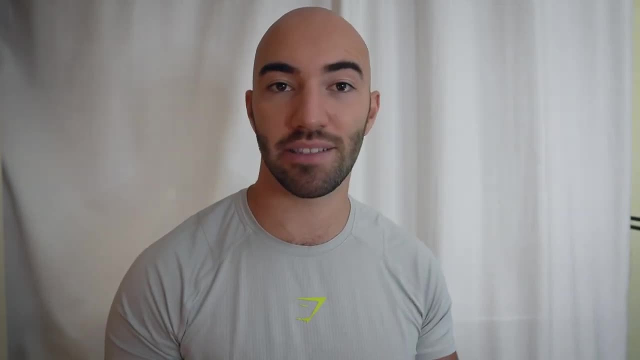 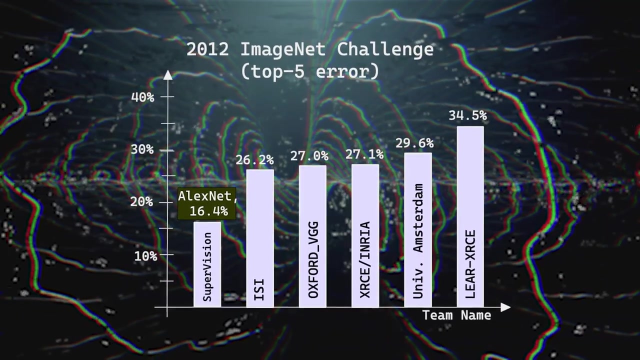 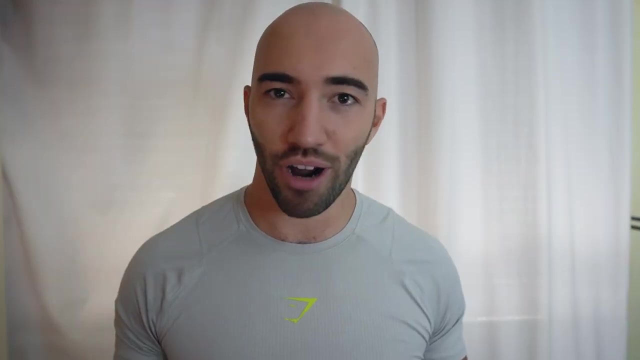 30th of September 2012, the latest challenge results were released, and one of those results was a lot better than any of the other results, and it came from a model that most people thought was just not practical, and that was AlexNet. AlexNet was the first model to 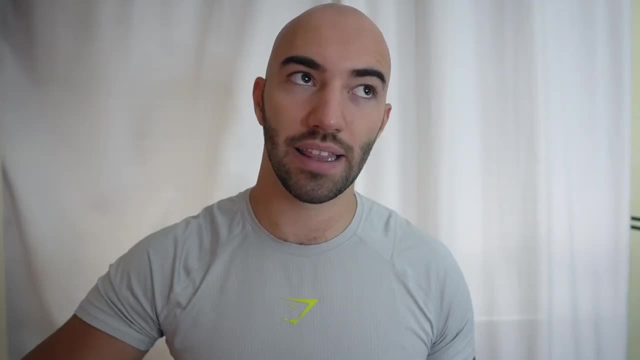 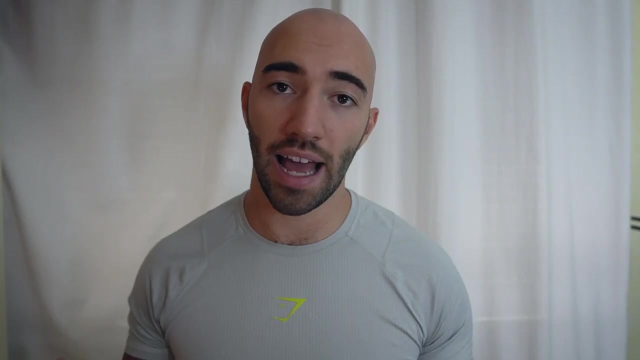 score a sub 25% error rate. and that same year the nearest competitor was a was nine point eight percentage points behind AlexNet, and they had done this with a deep-layered convolutional neural network which at the time people were not really taking seriously. now to understand AlexNet, it's probably best. 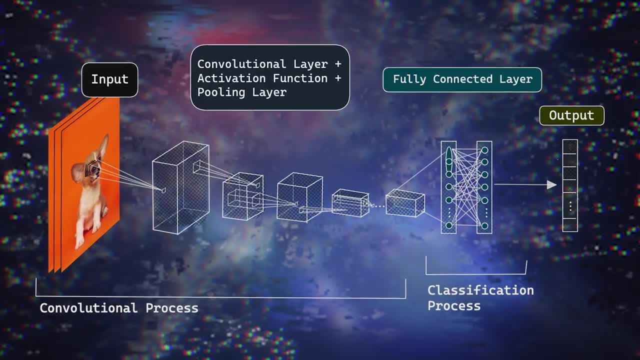 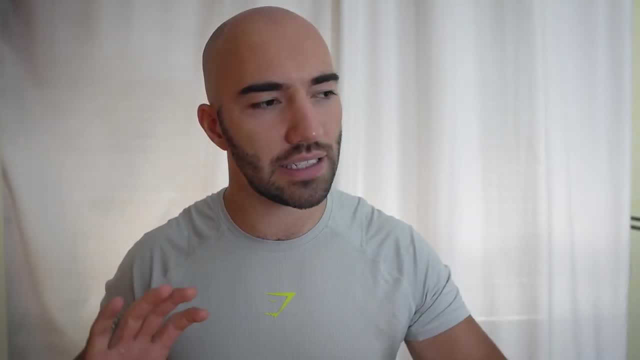 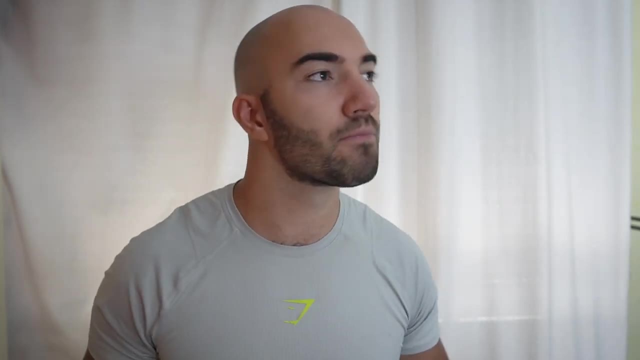 we very quickly cover a little bit of what a convolutional neural network at actually is. so convolutional neural network, or CNN, is a neural network layer that has a special layer called a convolutional layer, and today the these models are known for computer vision. they have been for quite a long time. 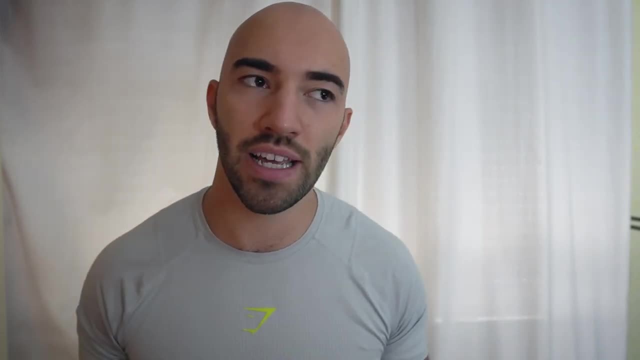 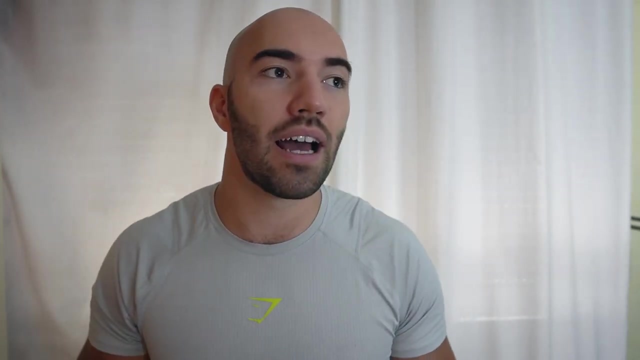 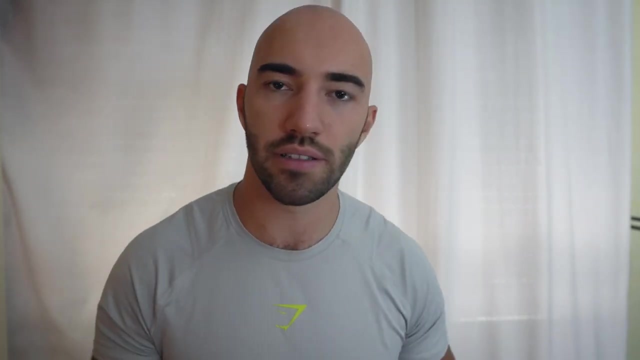 sort of undisputed champions of computer vision and actually you know that has changed a little bit and literally like the past couple of years, but right now that they're still pretty dominant and unlike a lot of the models back in 2012 and earlier, these did not need too much of manual feature. 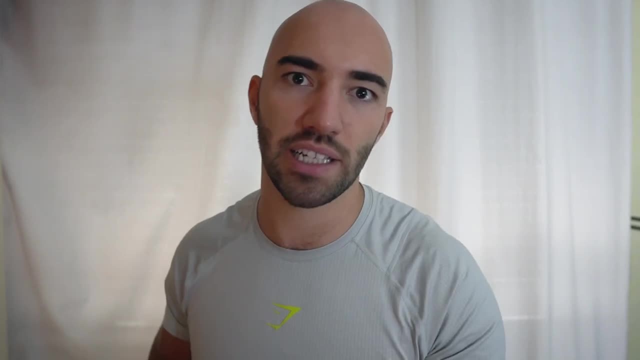 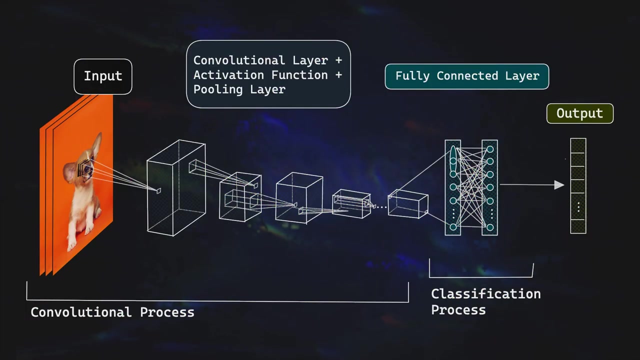 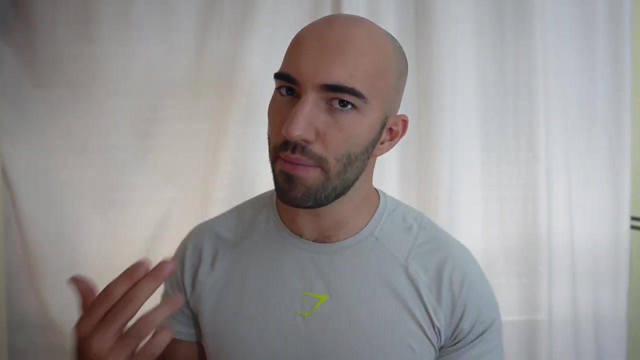 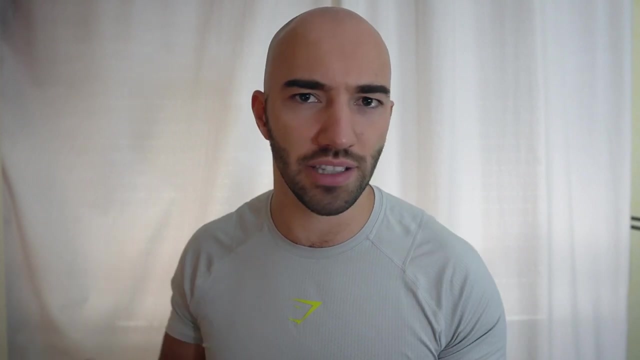 extraction or too much image pre-processing before feeding data into the model. they could just kind of deal with that themselves. CNN's use several of these convolutional layers stacked on top of each other and what you find is that the deeper the network is, the more the better it can identify more sort of complex concepts or objects in. 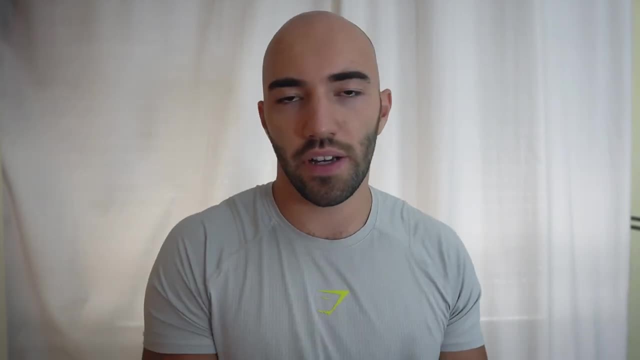 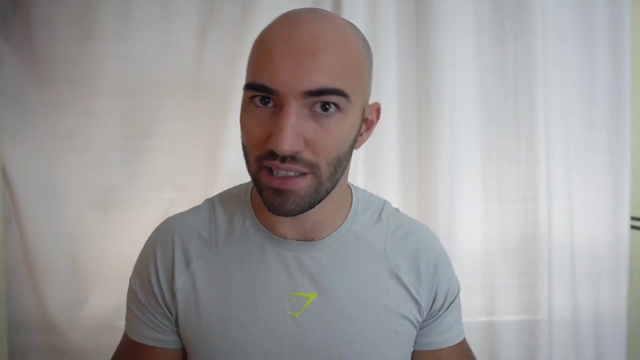 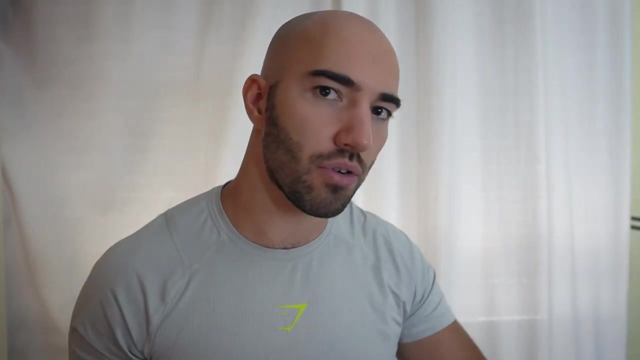 in images. so, for example, the first with the first few layers, you're probably going to just kind of identify: okay, this is an edge, this is a circle, maybe this is this shape and maybe some textures. as the network gets deeper and you add more layers to it starts to abstract those features and 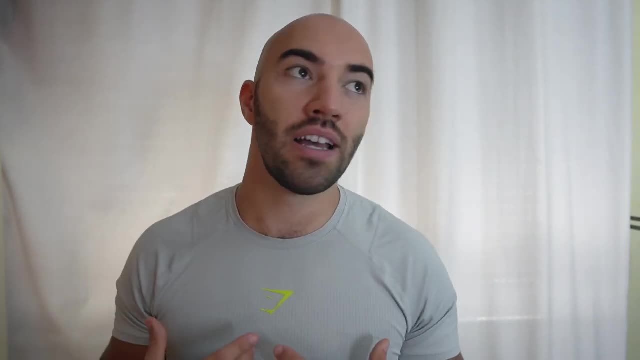 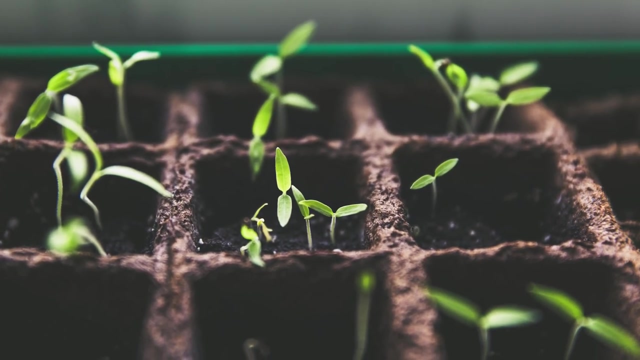 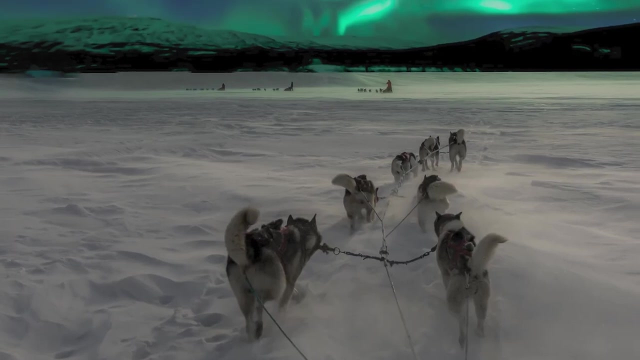 and identify more abstract ideas. So a deeper network will be able to identify. okay, this is like a living thing, And then you go, you build a deeper network and it can identify mammals, and then it can identify dogs, and then it can identify Siberian Huskies. 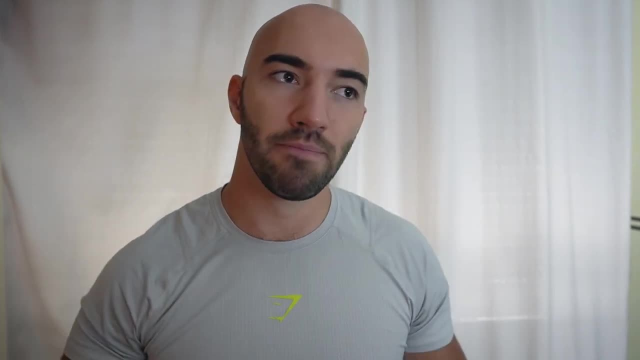 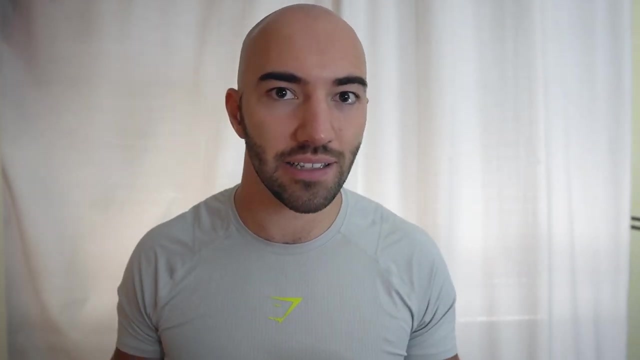 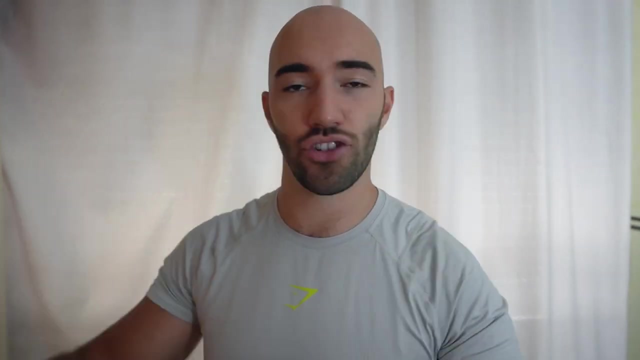 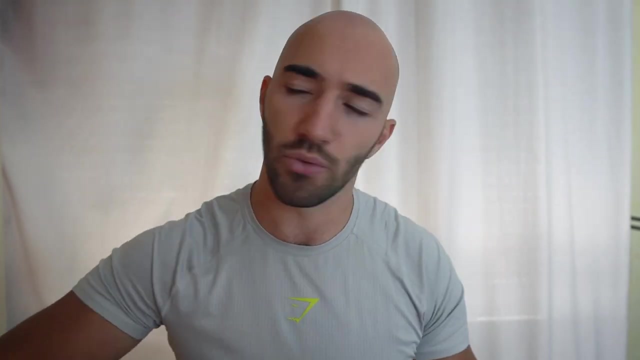 So as the model gets deeper, its performance and its ability to identify more nuanced things gets better. So at the time these models were overlooked because essentially to train these, to get good performance from one of these models, they need to be really deep. 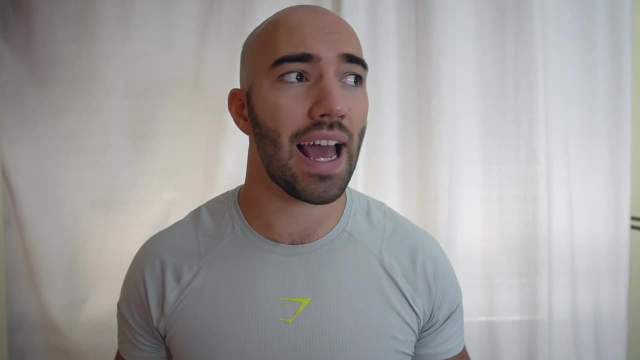 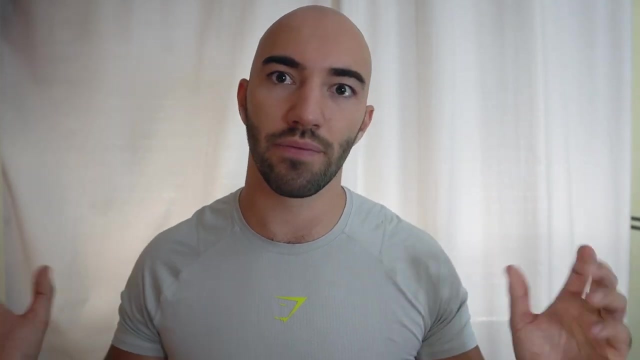 which means that they have a lot of parameters. okay, And the more parameters you have, the longer it's gonna take your model to train- If you can train it at all- if it's too big and doesn't even fit in the memory on your computer. 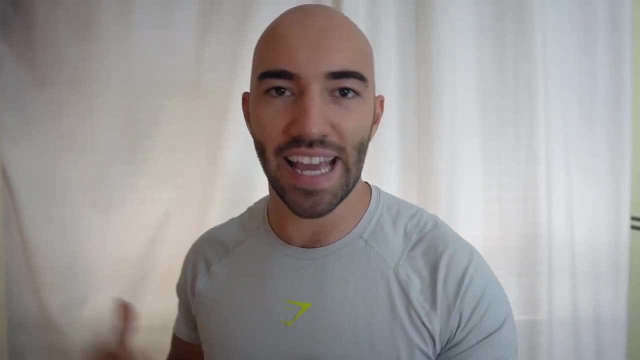 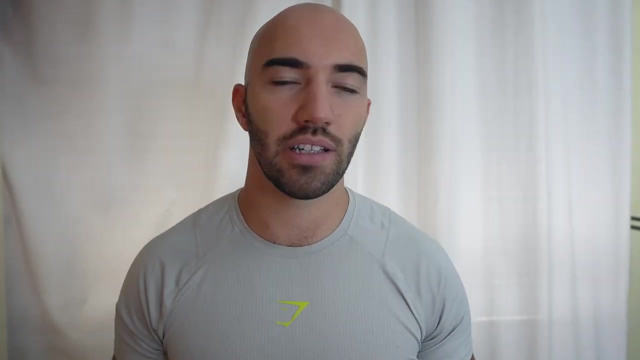 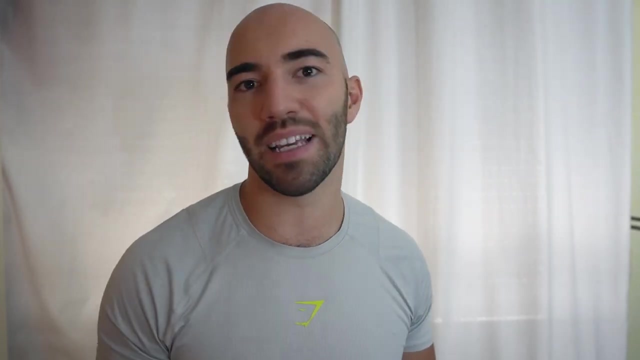 and also the more parameters it has, the more data it has to see before it can produce sort of any good performance of anything. As a result of this, they were simply overlooked. Yet the authors of AlexNet won the ImageNet Challenge in 2012. 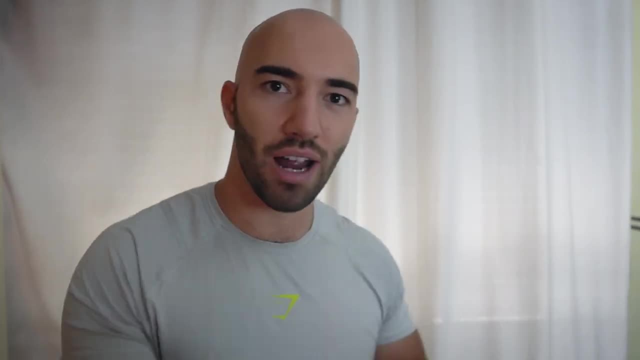 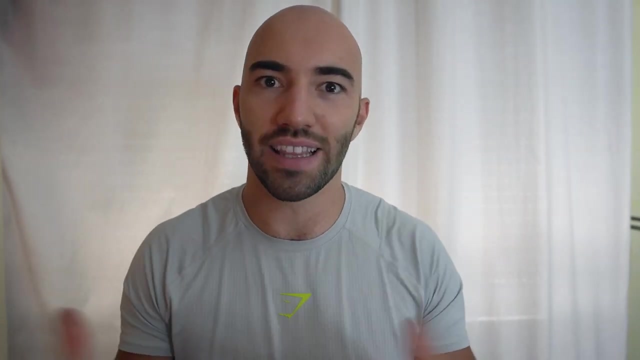 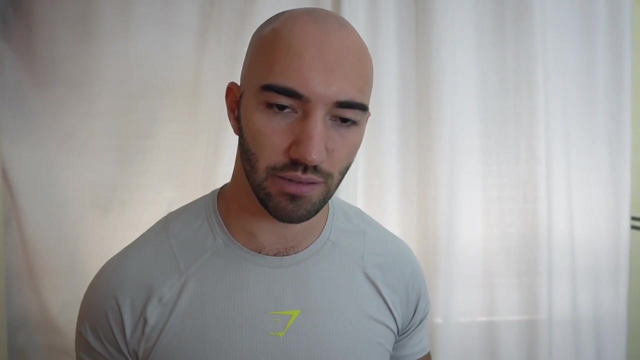 and it turns out that they were the right people in the right place at the right time. Several pieces came from different places to create this. ImageNet provided a massive amount of data needed to train one of these deep layered convolutional neural networks A few years earlier, in 2007,. 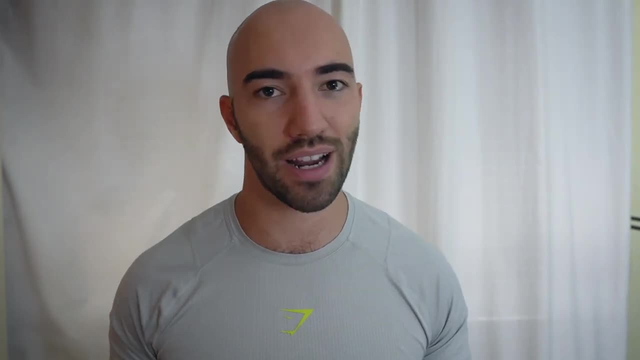 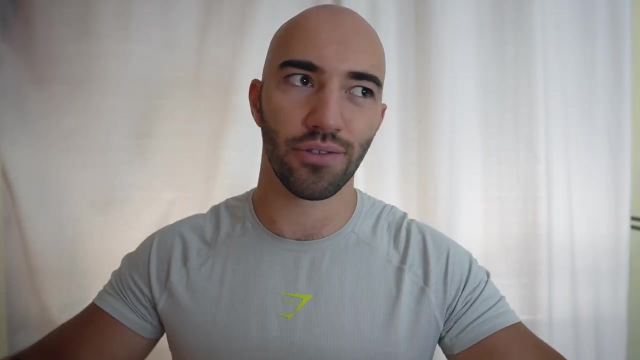 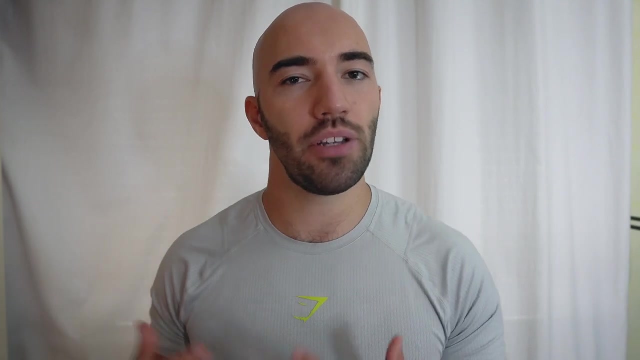 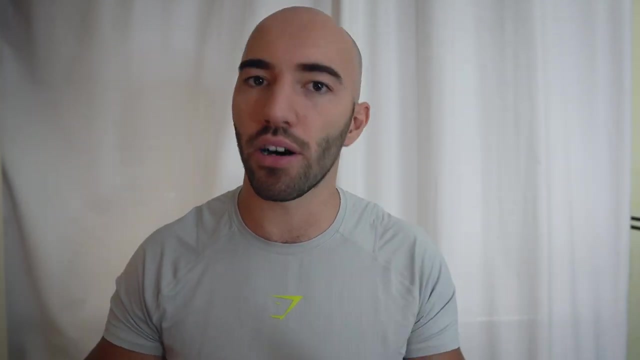 NVIDIA had released CUDA, which you may recognize the name of, So an API that allowed software access to the lower level, highly parallel processing abilities of CUDA enabled GPUs from NVIDIA, And GPU power in itself was reaching a point where this training, these big models, was becoming possible. 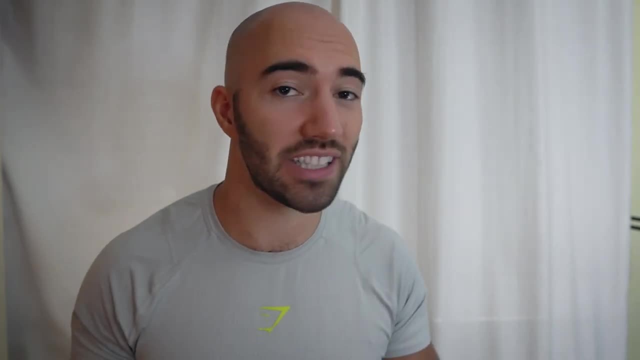 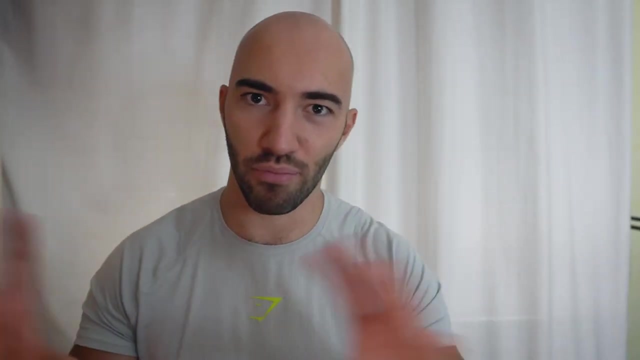 although it wasn't quite there yet at the time- for a single GPU. So AlexNet was by no means small, and because of that the authors had to solve a lot of problems to get all this working. So AlexNet consisted of five convolutional layers. 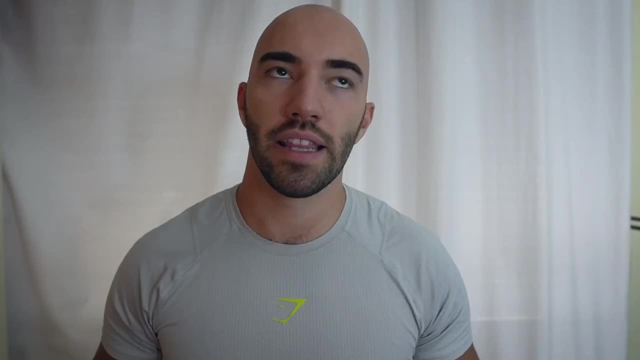 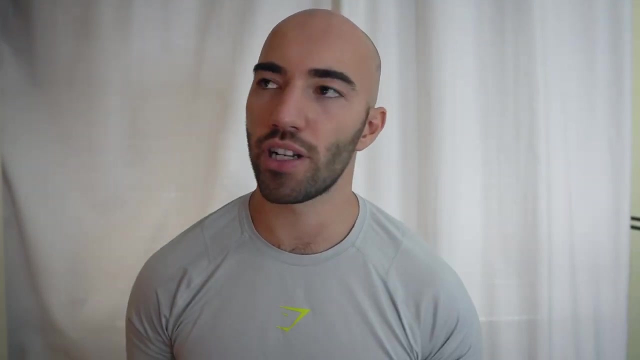 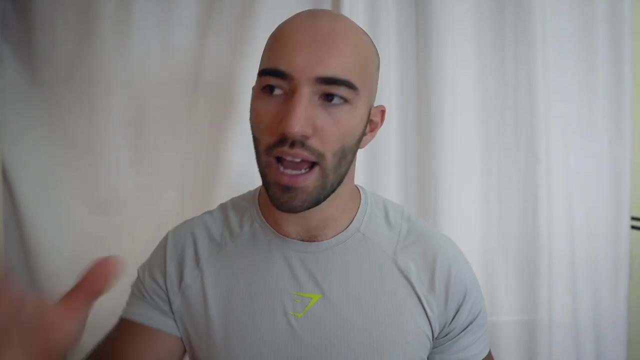 followed by three fully connected linear layers. The final layer to produce the 1,000, classifications required by ImageNet was a 1,000 node layer that used a softmax activation function to create this probability distribution over all of those classes. Now, a key conclusion from AlexNet was that 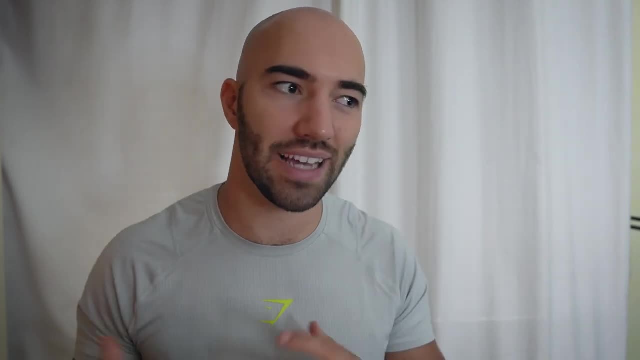 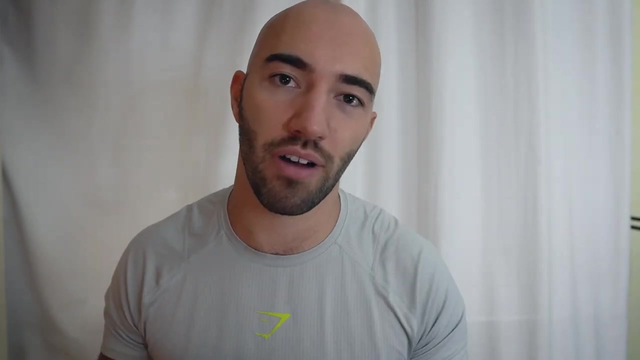 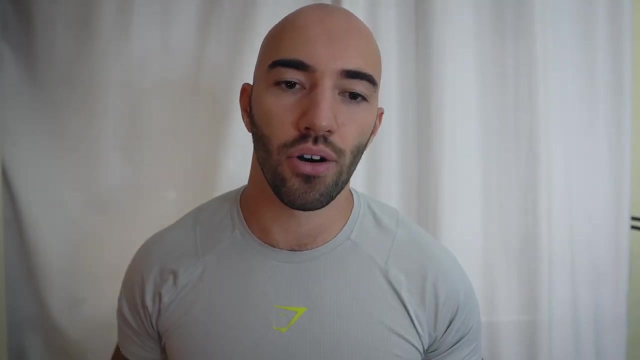 the depth of the network was key to getting the performance that they got, And that depth, as I mentioned before, it creates a lot of parameters that need to be trained, Making training the model either impractically slow or just simply impossible. 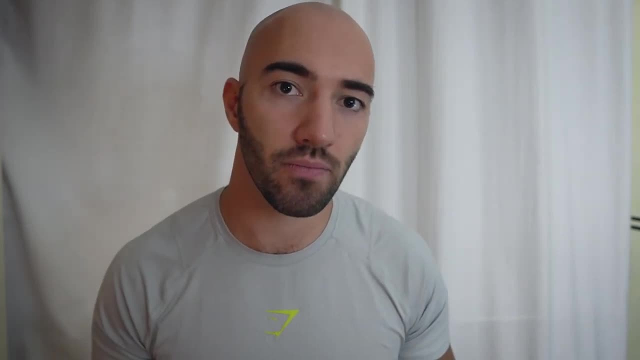 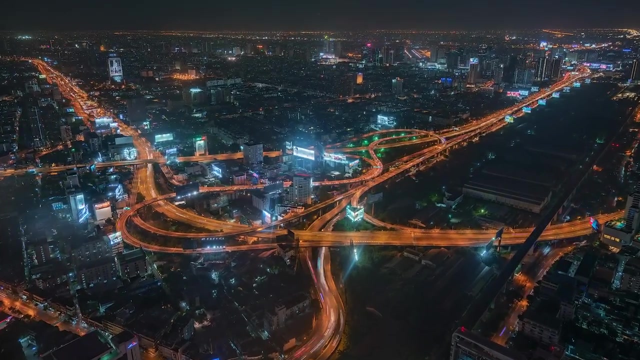 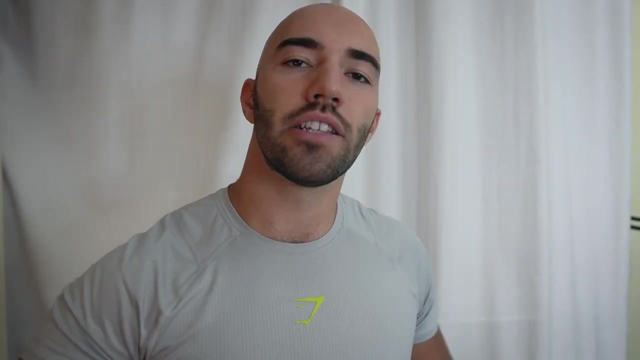 or at least that was the case if you were going to train it on CPU. So they had to turn to GPUs, but at the time the high-end GPUs only had a memory of about three gigabytes, which was not enough for AlexNet. 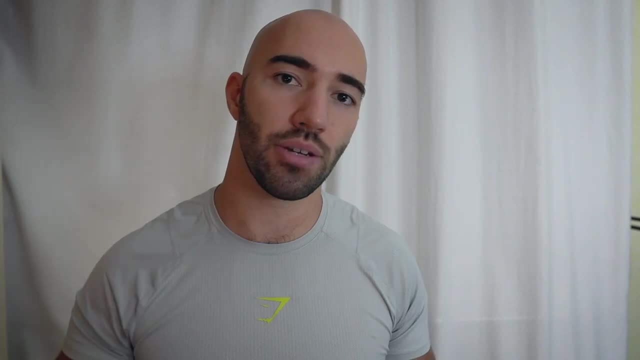 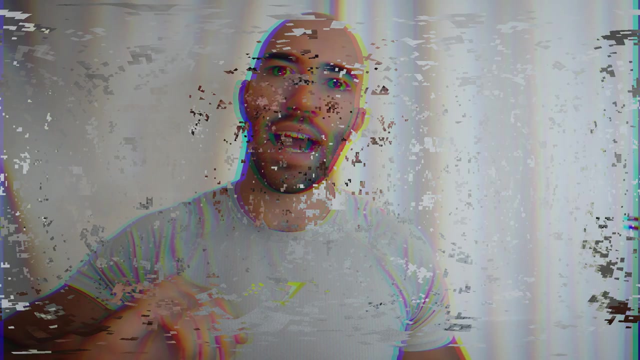 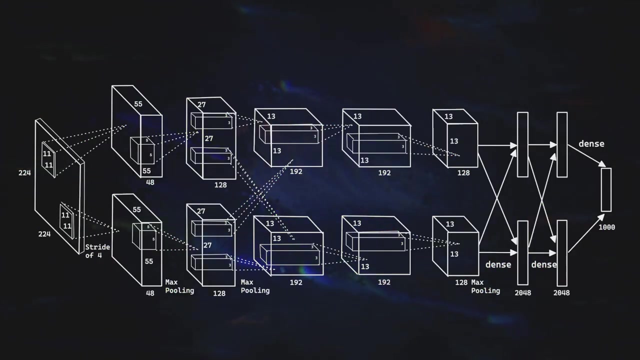 So to make it work, they had to distribute AlexNet across two GPUs, And they did this by pretty much splitting the layers in two and having half of the network on one GPU, half the network on the other GPU and having a couple of connections between the layers. 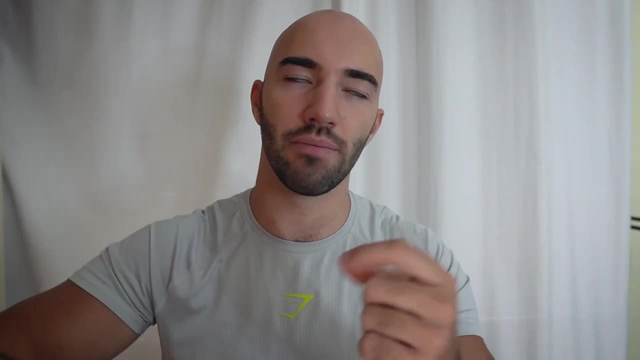 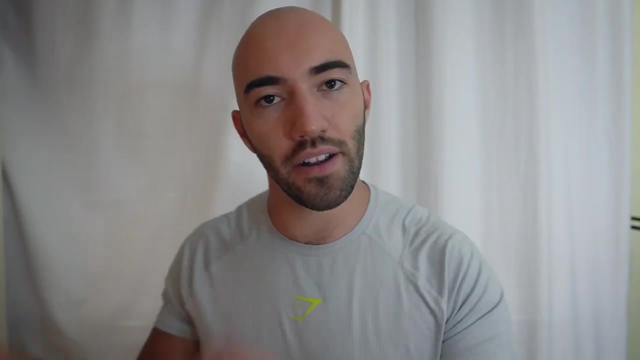 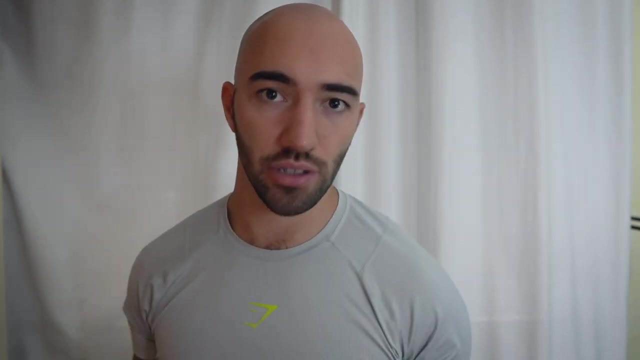 So they had a couple of points where the information could be passed between those two halves And then at the end they came together into the final classification layer. Another important factor is that they swapped the more typical softmax and tanh activation functions of the time. 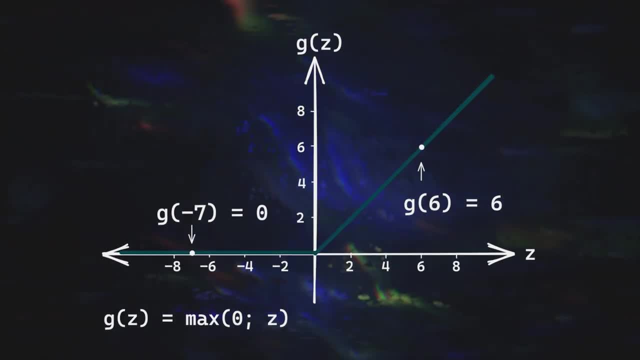 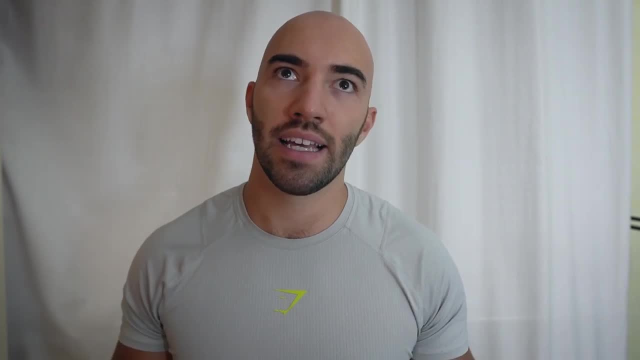 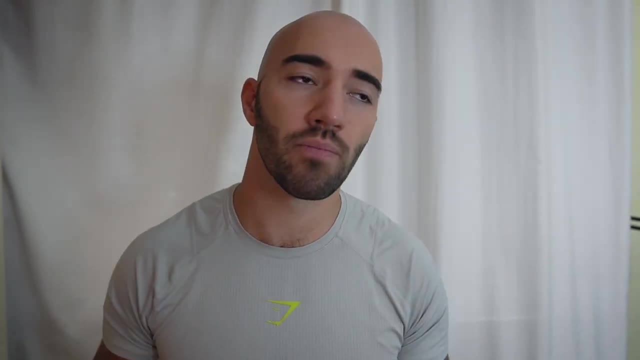 for a rectified linear unit or ReLU activation function, which again further improved the efficiency of the model and also meant that they didn't require normalization that you would usually have to do if you had tanh or softmax, because both of those activation functions over many layers. 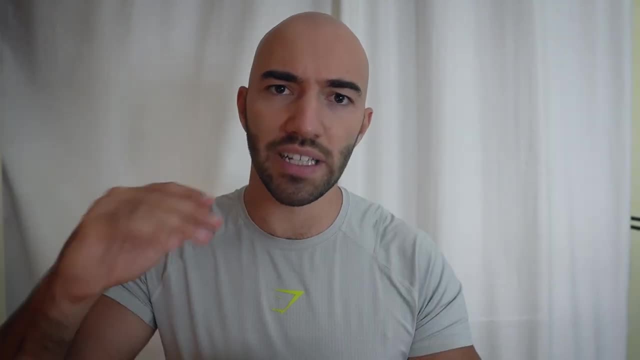 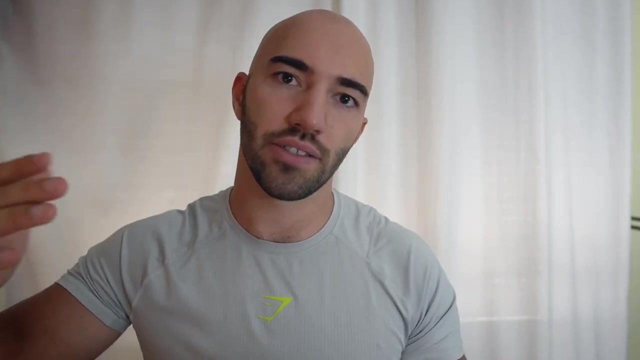 you can get what's called a saturation in your activations, which means the activations in your, in your neurons either kind of push towards the two limits of one of those activation functions. So for example, with softmax you'd end up all your activations. 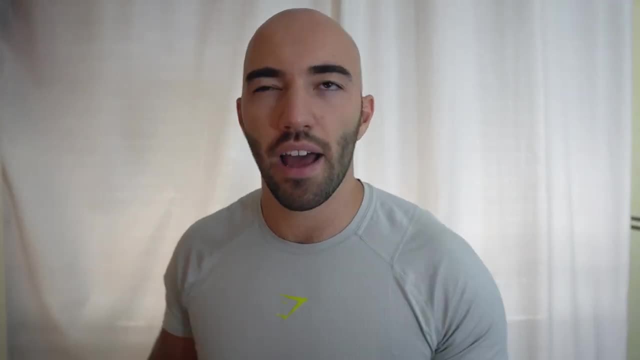 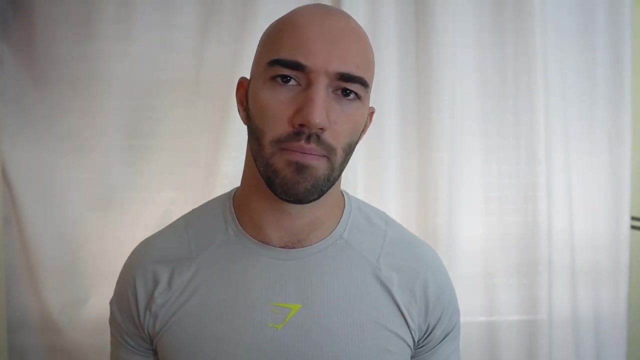 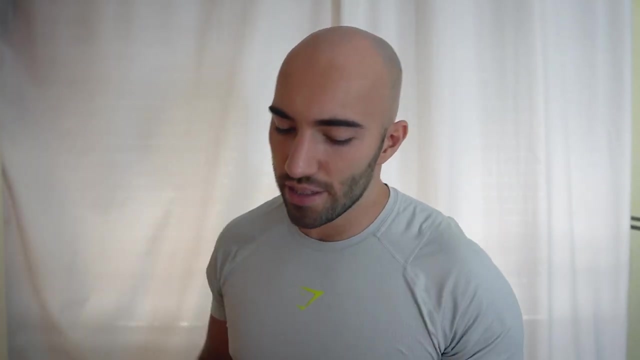 be pushed towards a one or zero. Nonetheless, they did use another type of normalization called local response normalization, but that's not really used anymore. Nonetheless, for AlexNet that was still a critical component. Now, another super important thing that is still used today: 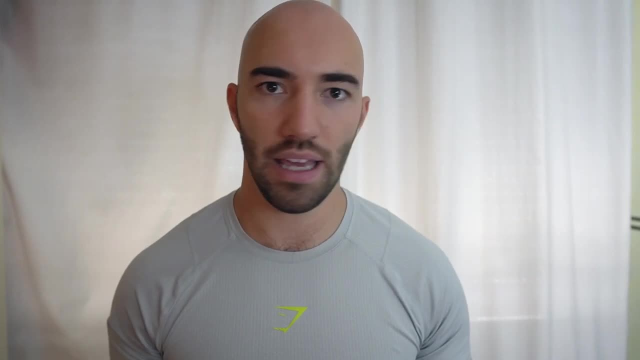 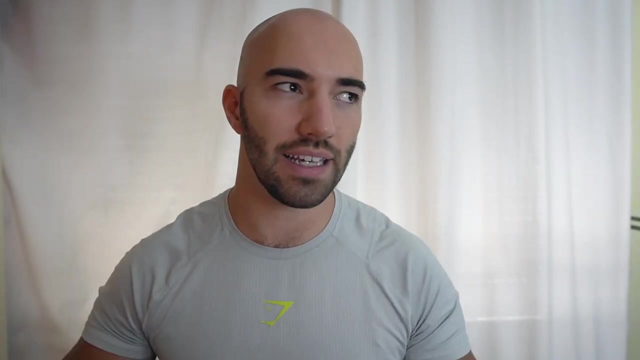 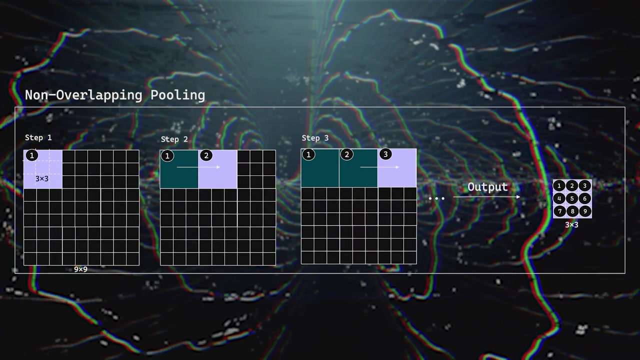 that AlexNet introduced was the use of overlapping in the pooling layers. Now pooling is already used in convolutional networks and it essentially just summarizes a window of information from one layer into a single activation value in the next layer. Now overlapping pooling does the same thing. 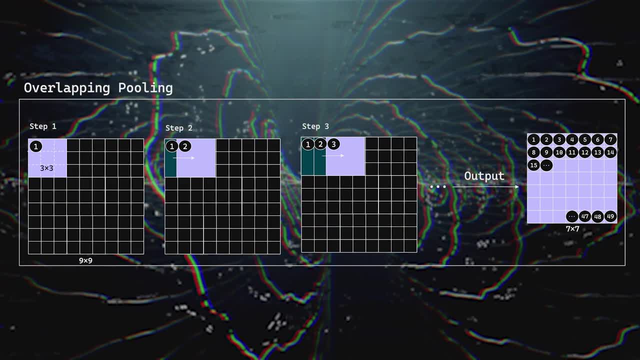 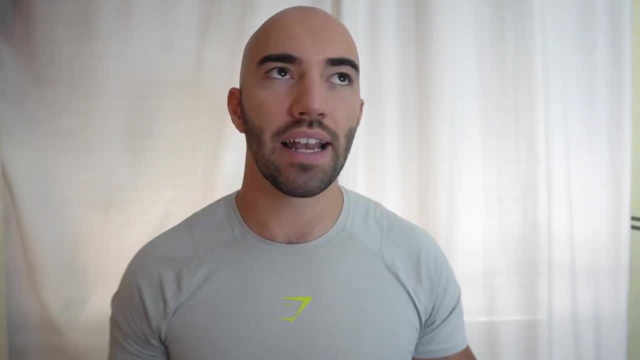 but there's an overlap in the window that gets passed along in the preceding layer, So there's always it always sees a little bit of the previous one. There's always an overlap in the previous window. okay, And they found that this reduces overfitting of the model. 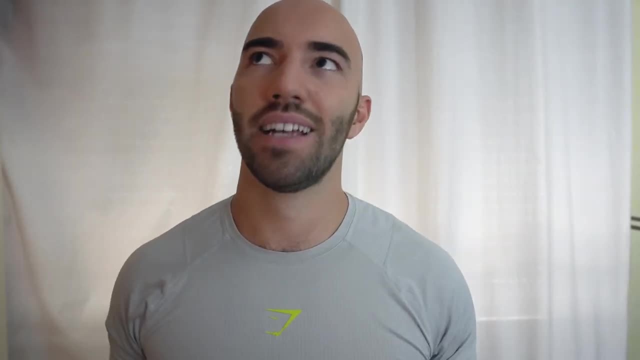 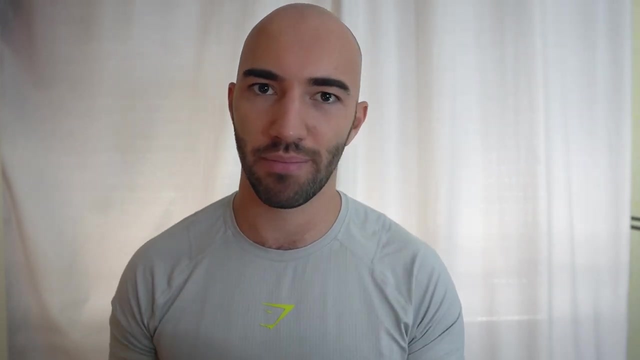 and improves the performance. So that is how they got AlexNet to work and a few of the details behind. actually, you know how it worked and why it worked so well at the time. Now I think it's great to talk about all of this. 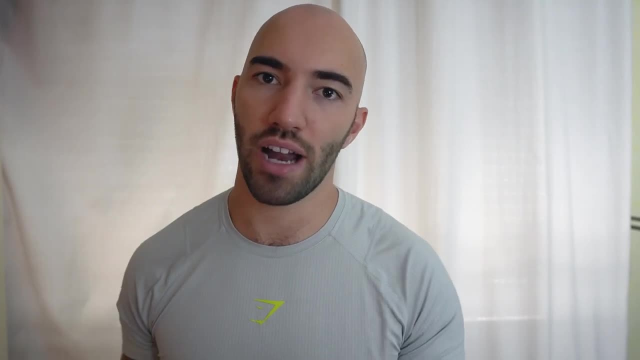 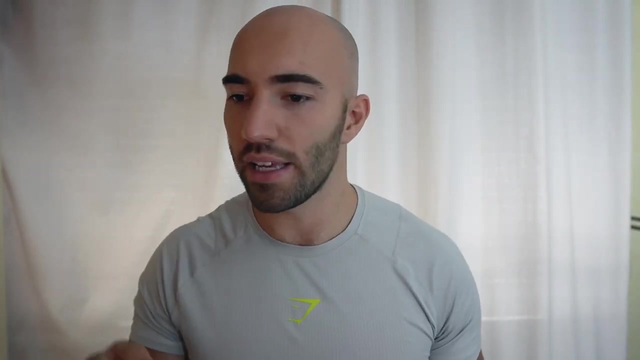 but, as I said at the start, I think it's better to go through everything or back everything up with a little bit of code. So we'll go through. So we've got a notebook that you can find a link to the Colab version of this notebook. 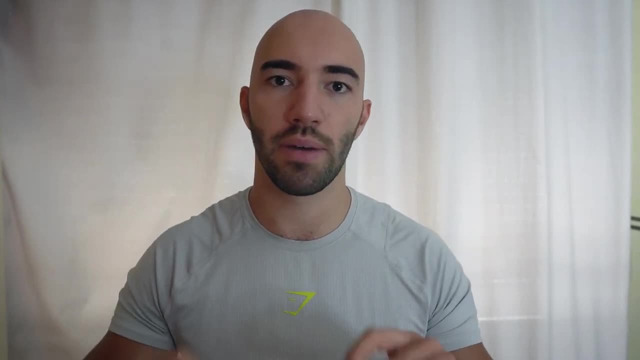 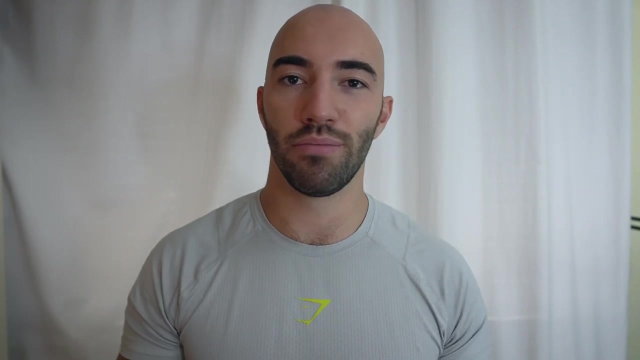 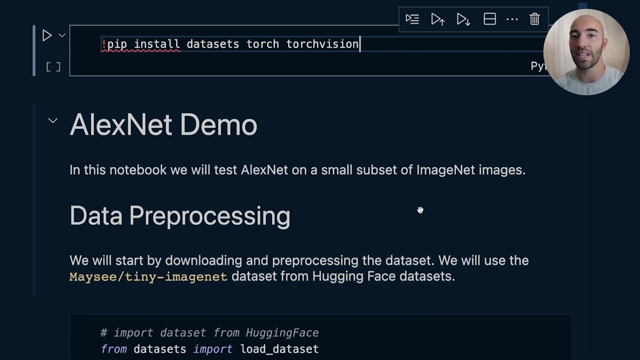 in the description below, or if you're reading this on the Pinecone article page, it will be in the resources section at the bottom And, yeah, we'll start going through that. Okay, so we're gonna start by downloading and pre-processing our ImageNet data set. 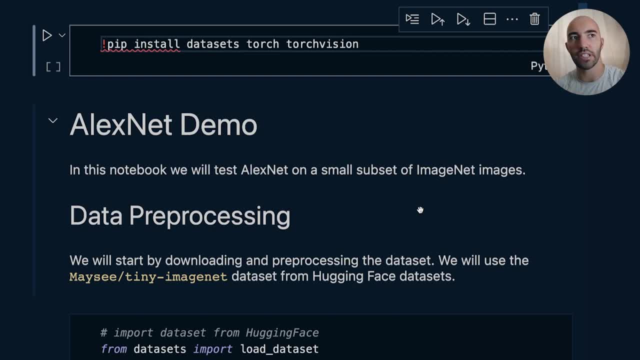 So we're not using the actual ImageNet itself. We're using another hosted version, a version of ImageNet which is much smaller that we can find on Hugging Face. So to use this we will need to pip install a few things. 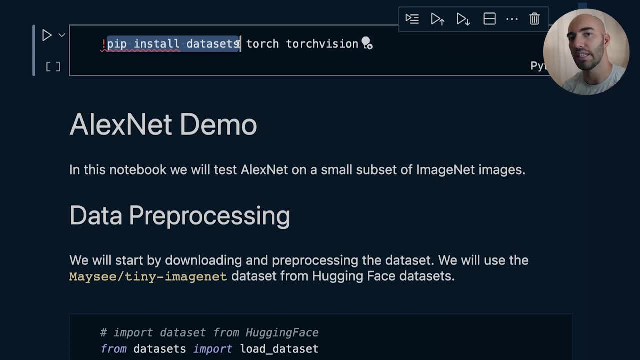 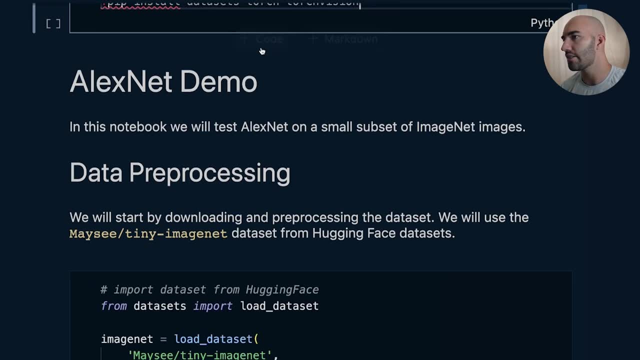 So, pip, install data sets, which is how we're gonna use the ImageNet data set, And later on we're also going to be using Torch and TorchVision, so install those as well. So this is the data set we're gonna use. 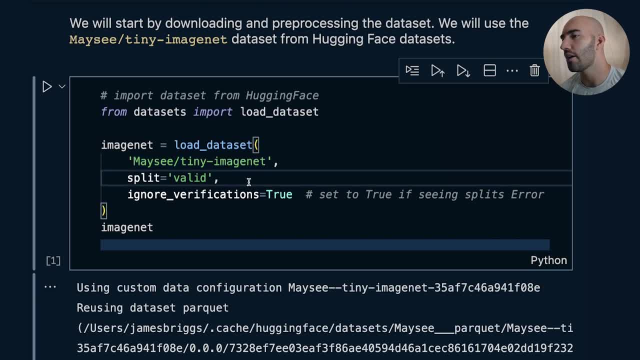 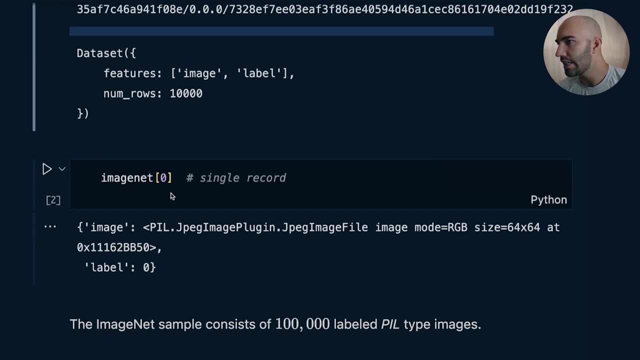 So we're using this Macie tiny ImageNet data set. Now, this is a validation, This is a validation, This is a validation split And that contains- I think it's 10,000, we can see here: yeah, 10,000 labeled images. 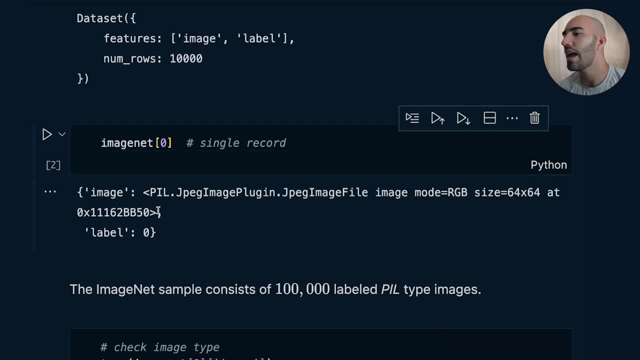 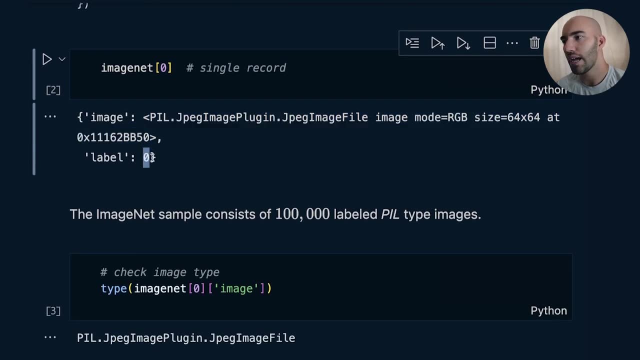 Okay, and then we can see a single record in there. So we have: every image is stored as a pill image object and they have these labels. So this one has labeled zero. We don't necessarily know what that means right now. 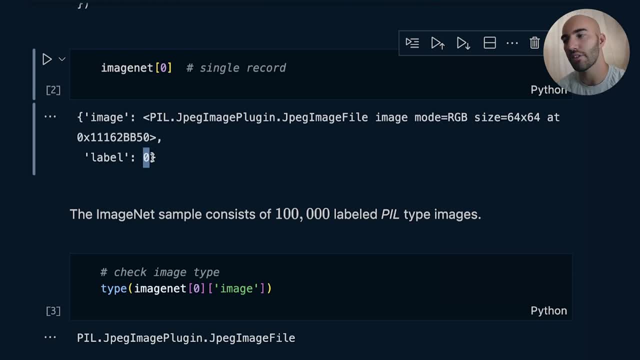 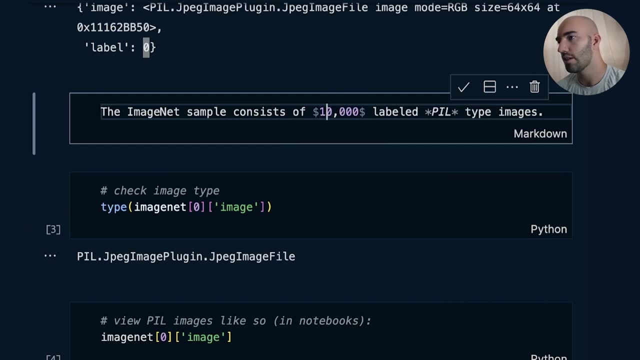 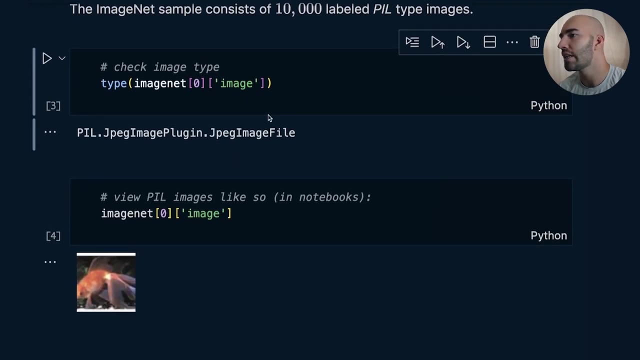 but later on we'll see how we can actually figure that out. So this one's referring to the actual training data set. So the training split of this data set does contain 100,000 of those labeled images. Now we can check the type. 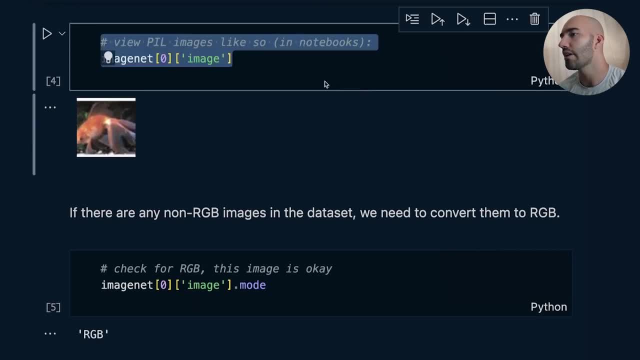 It's the pill object and we can see. okay. So when we're in a notebook like this, we can just call this ImageNet and this is just how we show that in the notebook, So we can see it's a goldfish. 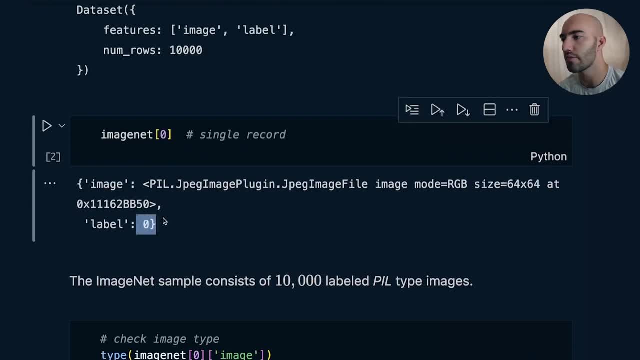 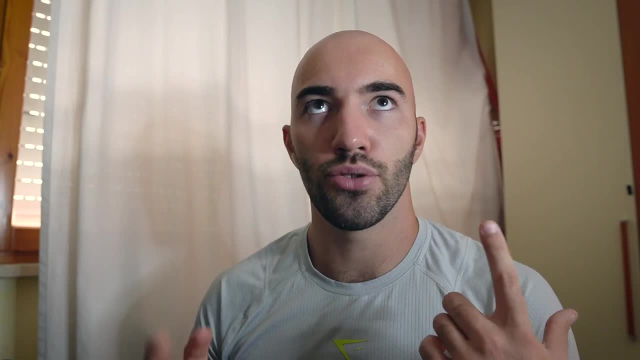 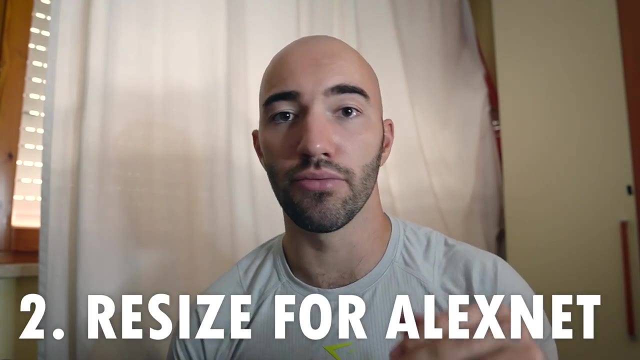 So we can probably guess that labeled zero actually means goldfish. So there are a few pre-processing steps that we need to go through. So we need to convert all images into an RGB format, So it will have three color channels. We need to resize all these images. 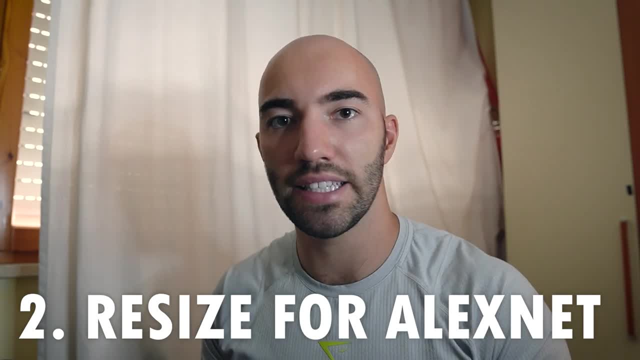 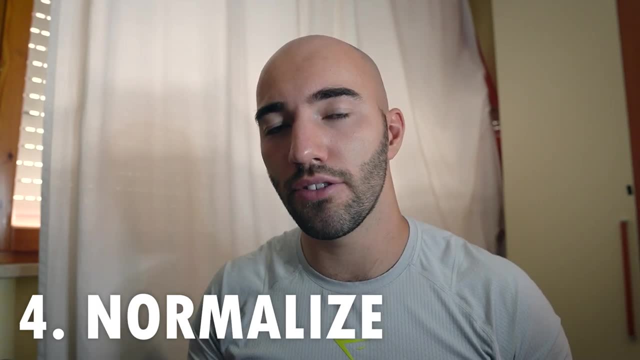 to fit the expected dimensions of AlexNet. We need to convert into a tensor for PyTorch. We need to normalize those, those values and stack. So when we have multiple images, we're gonna stack them all into a single tensor, okay, 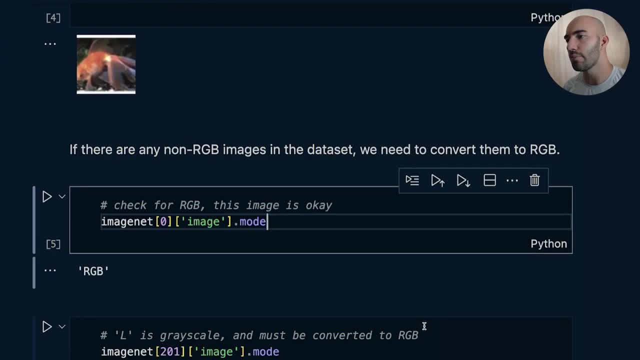 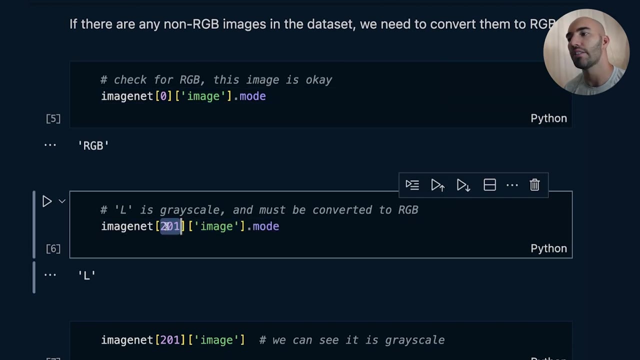 It's to create our batch, So we start with RGB. AlexNet, as I mentioned, assumes all images have three color channels: red, green and blue, But there are many other formats that are supported by pill objects, So we'll see here that we have grayscale, okay. 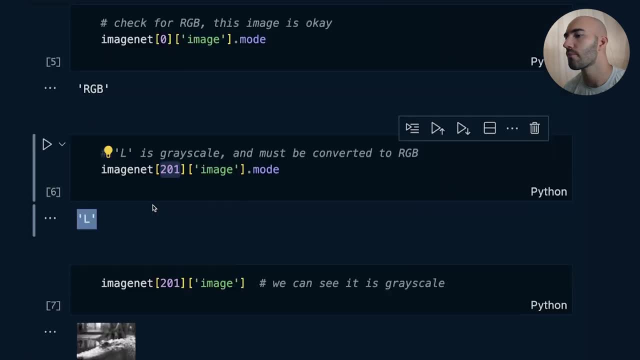 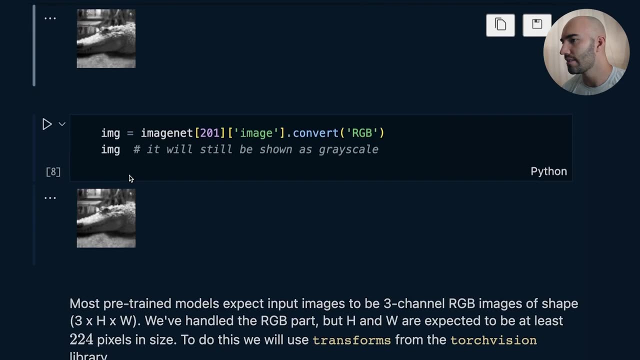 So this is 201.. This is a grayscale image because we have this L. There are other formats as well, so you need to be aware of those And we can see. I think it's an alligator. Yeah, an alligator in grayscale, okay. 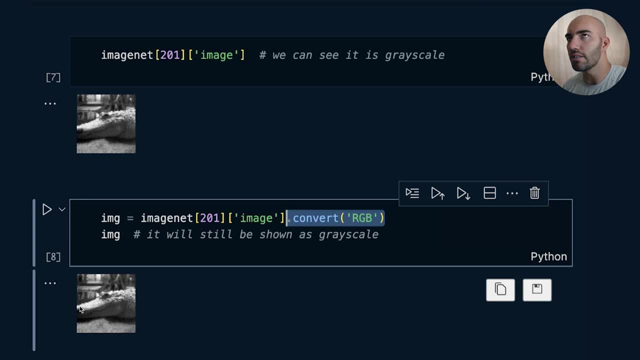 So we convert it into red, green and blue and we'll see: okay, it's still grayscale, That's fine, It will still be shown as grayscale, but in reality this only has one color channel, which is actually just like a brightness channel. 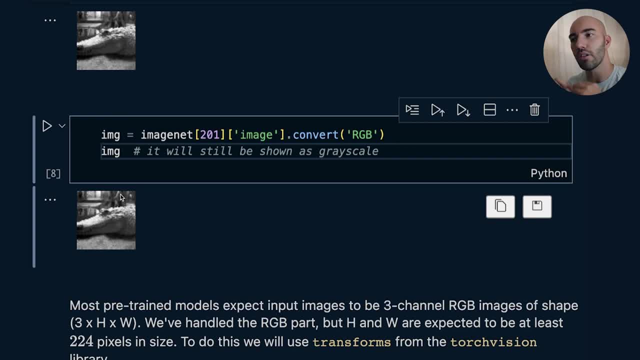 whereas this now has three color channels: red, green and blue- but they're all of equal values across those three channels, so it actually still shows as being grayscale, even though it is in a RGB format. This is how we handle the RGB part. 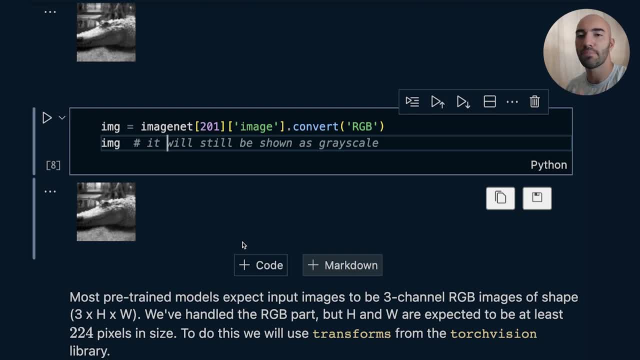 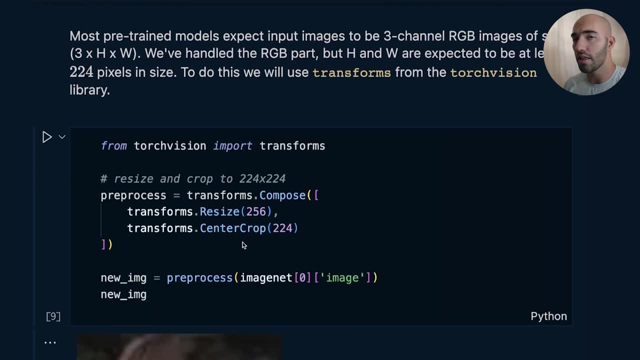 but we also need to resize the image to fit the expected dimensionality for AlexNet. So for AlexNet and for a lot of other computer vision models, the height and width of the input image is expected to be at least 224 pixels. 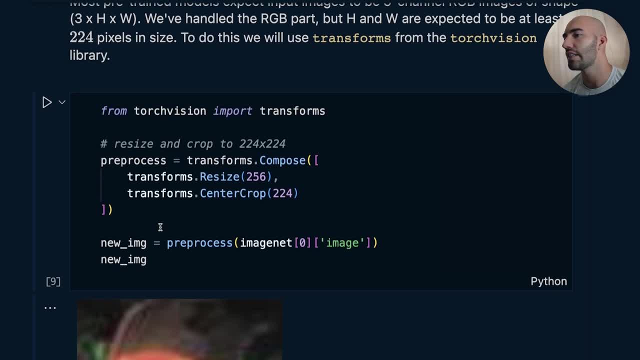 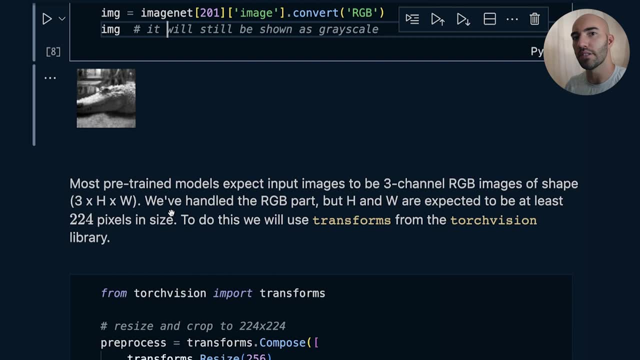 So we need to do that. We can by using this. So we're going to: first we resize the images, because these are very small images and they're not necessarily all going to be the square that we need, the 224 by 224.. 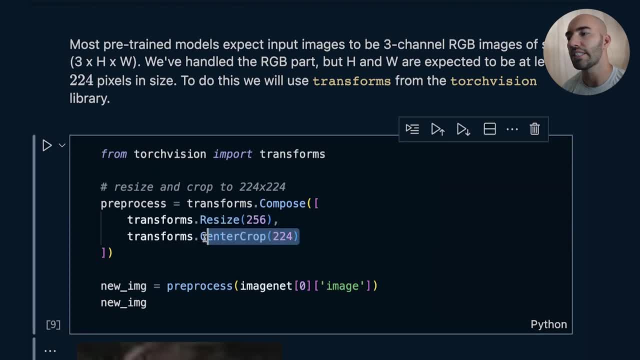 So we resize them to be bigger and then we use a center crop to crop out any edges and make sure that it is now square. So it's a square image of that dimensionality. And yeah, we're doing that. using this transforms function. 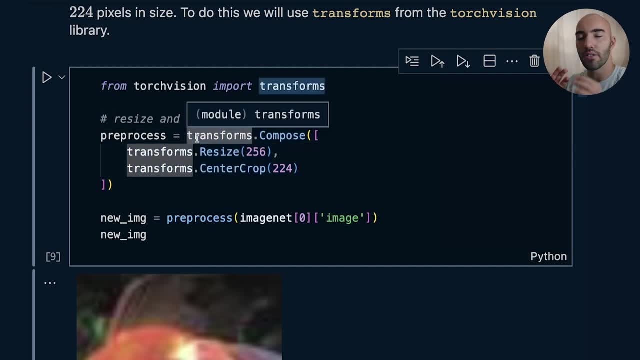 from TorchVision, which is a very good way of pre-processing your image data. It has a lot of functions and we'll see we'll use a couple more of those very soon. So if we have a look at our first image, 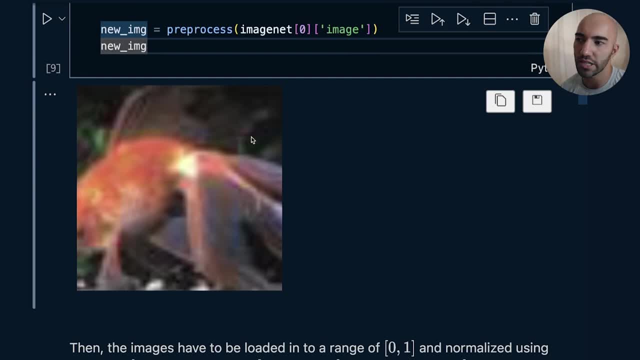 the goldfish image we see. it's now a bit bigger and we can also see it's kind of cropped, some of it as well, but we still get the. you know, we still get the idea of what is in that image. 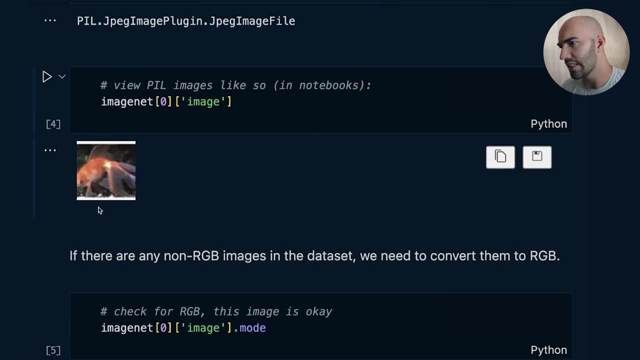 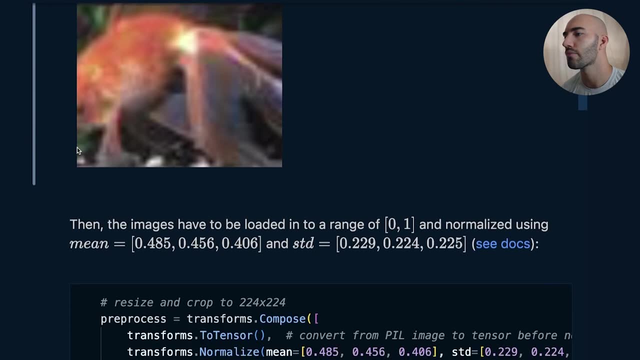 So if we compare that to this, here we can kind of see its eye at the front, there more of its head, whereas here it's kind of almost chopped off. Now, another thing we need to do is normalize all the values in these images. 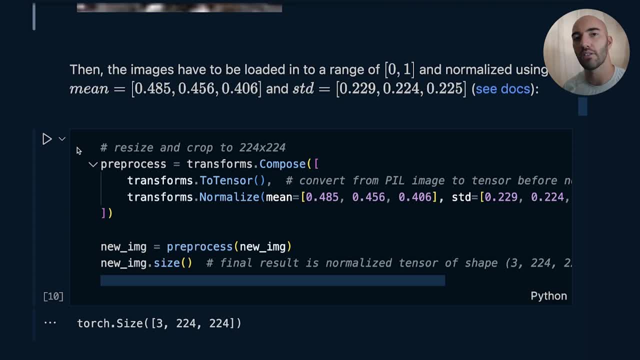 So RGB arrays tend to be in the range of zero up to 255.. And we need them to be in the range of zero to one And we need to normalize them using these values that you see here. So this mean of 0.4.. 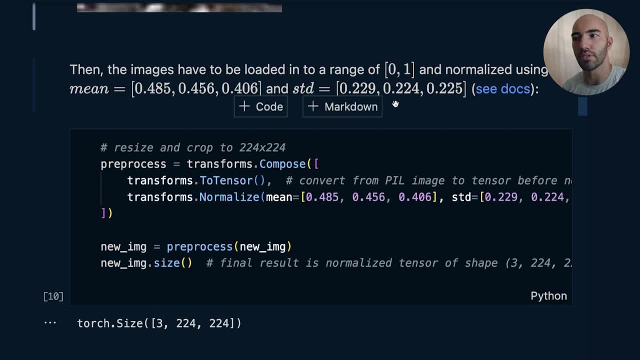 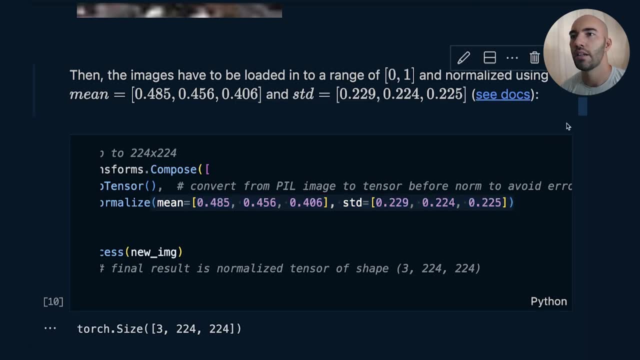 And so on, and the standard deviation is 0.2 and so on. This is specific to the AlexNet implementation from PyTorch. So we go on the AlexNet PyTorch page, you can go down and it. here we go. 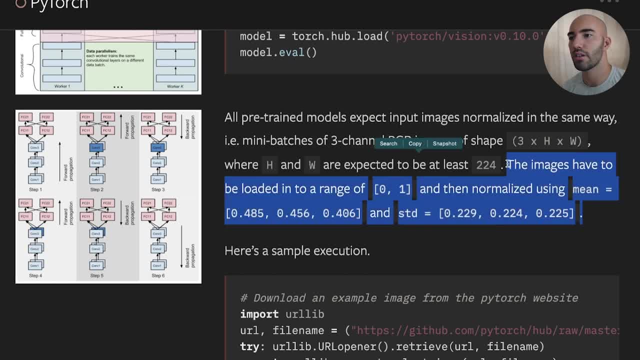 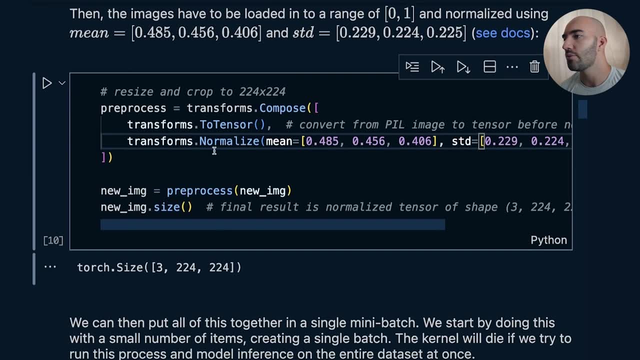 So the images have to be loaded into a range of zero to one and normalized using the values I just showed you. So that's why we're using those. And yeah, so we create this process function and then we process our images. We process our image through it. 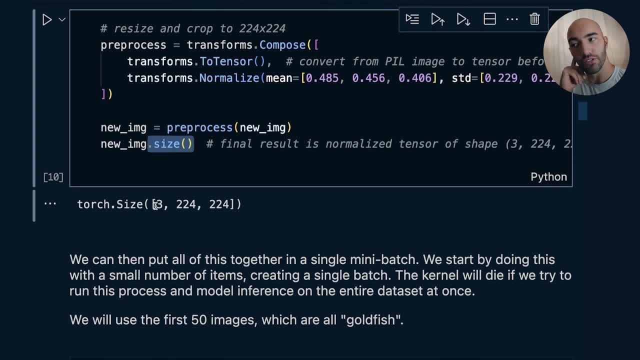 and then we can check the size. So the final result here is going to be that normalized tensor that we want and it's in the correct. it has the correct dimensionality that we need as well. So, yeah, that's perfect. Now we want to pull this together. 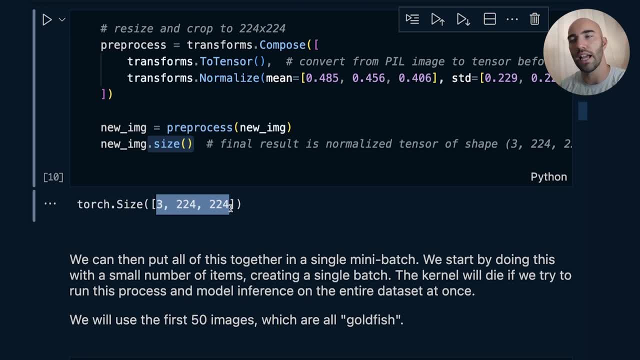 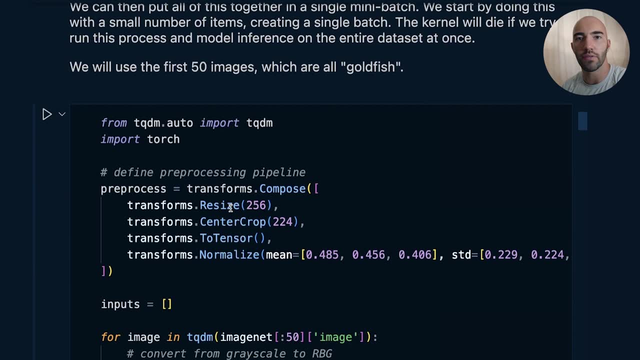 and we don't want to do it for every single image like this. We're just going to put it all together for a mini batch of images. So we're going to go with the first 50 images, because they're all goldfish and we can easily check the AlexNet's performance. 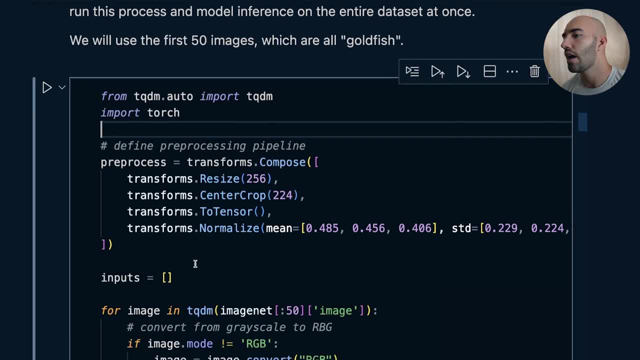 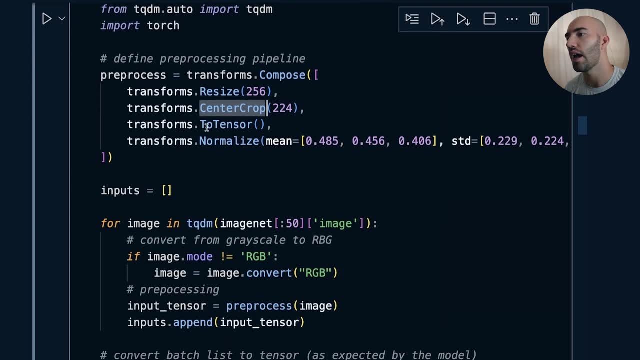 on that single object. So I'm going to redefine that pre-processing pipeline using everything we've just done. So we'll resize, we crop it to tensor. We have to do this, by the way, because PyTorch is expecting a tensor object. 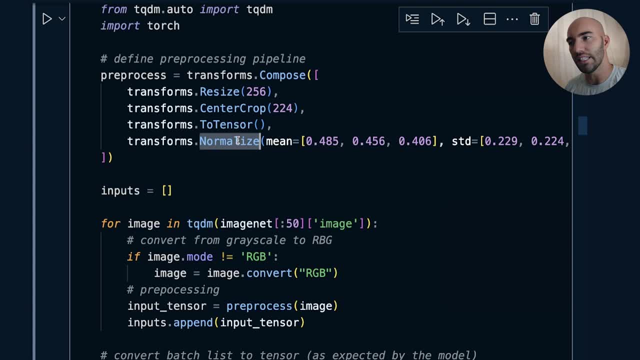 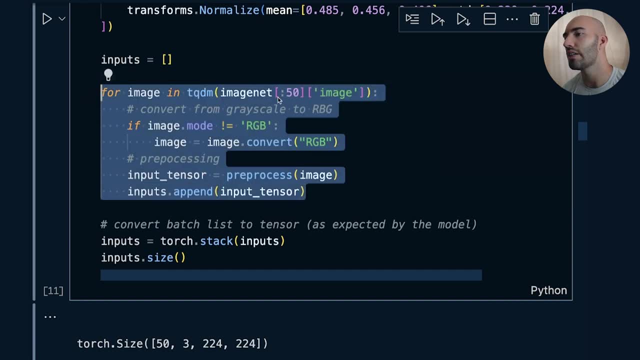 and before we normalize it it needs to be in that tensor format, otherwise we're going to get an error And then, yeah, we normalize it. So we go through every image in the first 50 images and we first convert any that are gray scale to RGB. 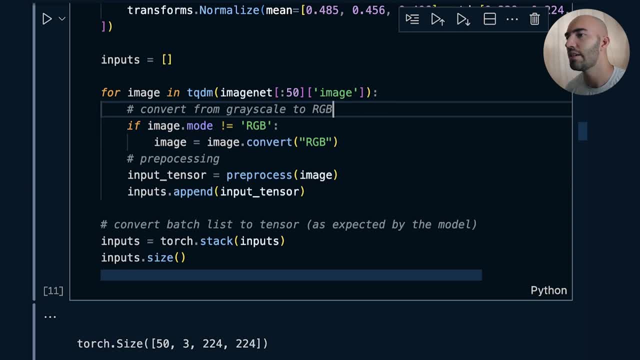 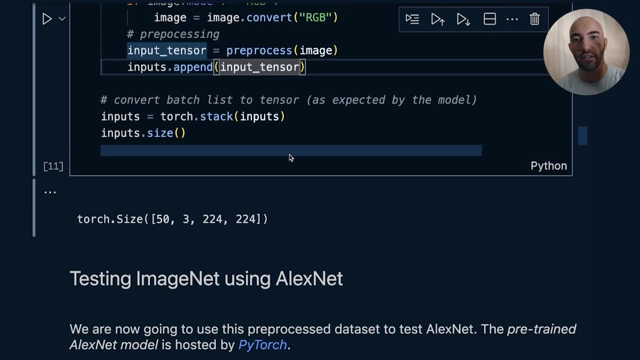 not RBG RGB- and we pre-process them, okay, And just append them to a list. Now that list, we want to stack all those together into a single tensor, So we do that here and we get this final mini batch of our images. 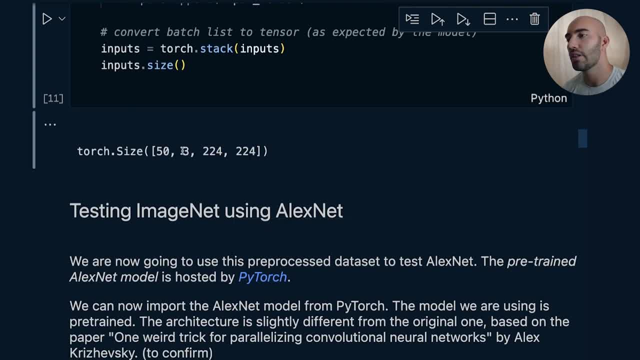 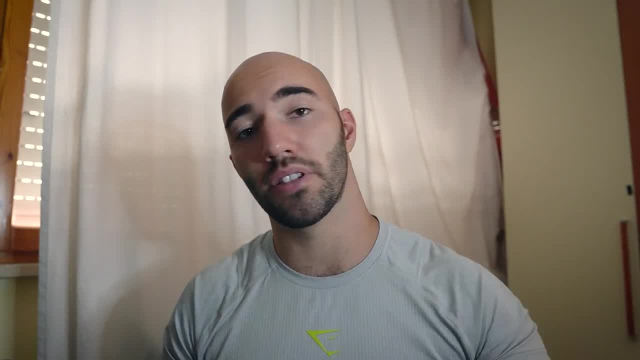 So we have a mini batch of 50, and we have those images that you can see with the dimensionality here. So with all of that done, we're now ready to move on to the inference step, So the prediction of the class label. 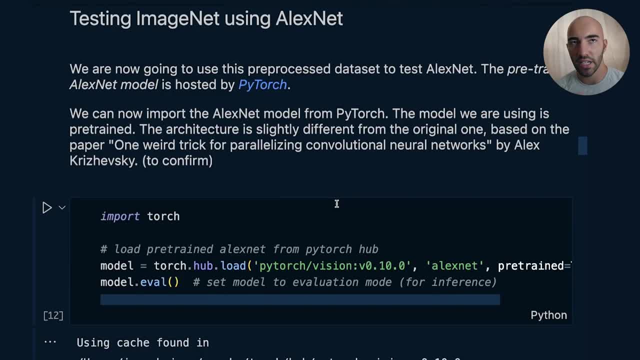 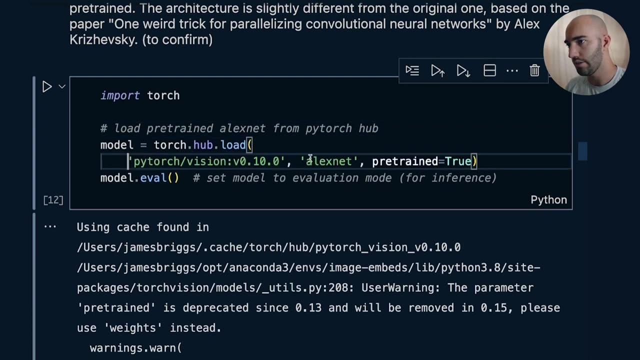 is for our images with AlexNet. So the first thing we're going to want to do is download the model, which is going to be hosted by PyTorch, So we can do that here. So let me, so you can see a bit better. 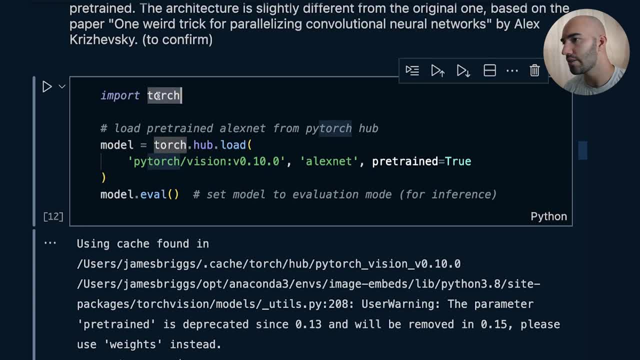 We import Torch, the PyTorch, and we just do Torch Hub load. okay, PyTorch Vision, let's just see the version that we're using. And then we have AlexNet and we're not going to train AlexNet. 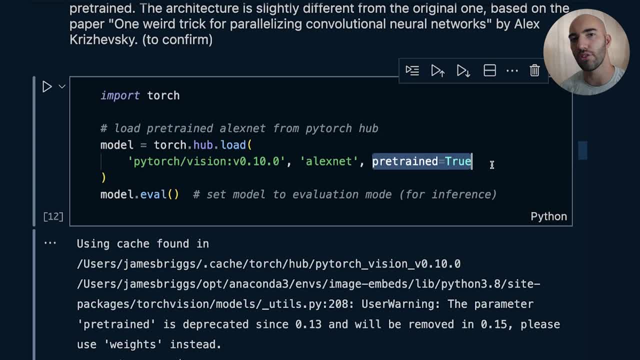 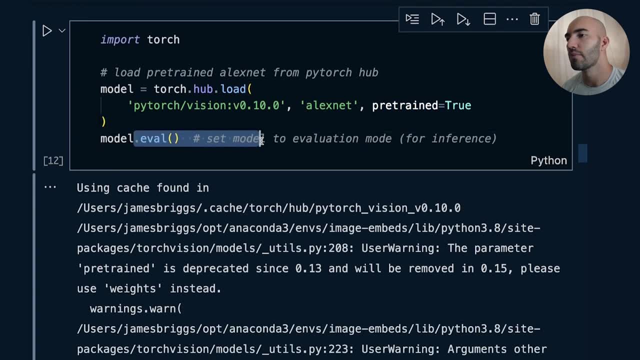 It would take a bit of time. So we're going to use a pre-trained model: weights. So this version of AlexNet has already been trained, And then we just say it's evaluation mode for inference. So for the predictions we don't want to train it. 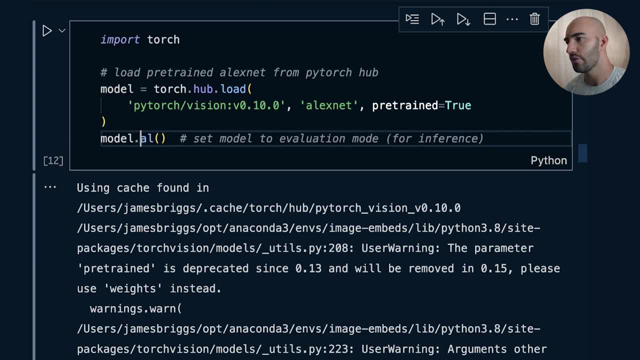 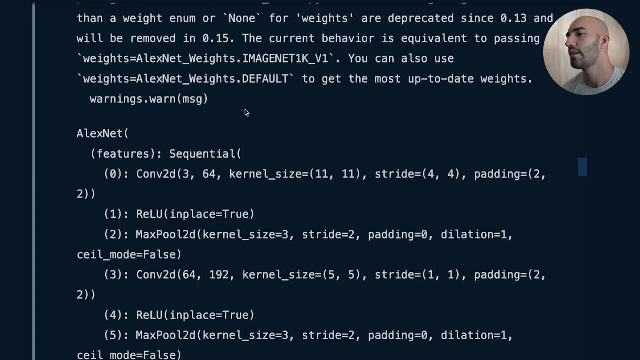 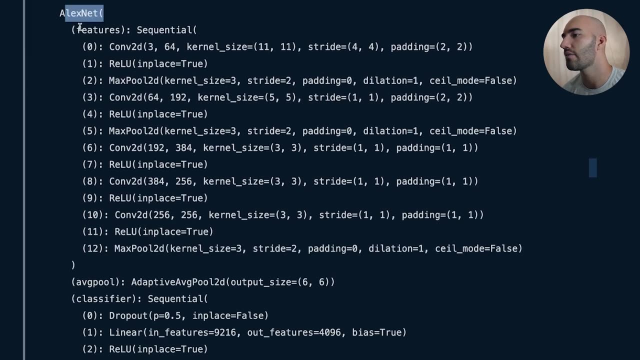 By default. I think it is in train mode, which looks like this. We want it in evaluation mode And then we can see the model structure here as well. So you can see AlexNet we have. So this is where we're creating the image features. 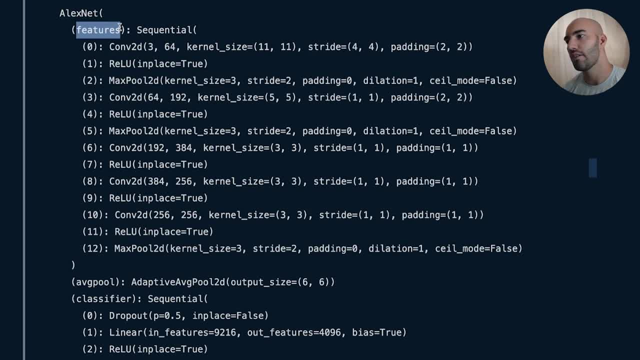 So there's many of these convolutional layers, followed by the radioactivation function, followed by the max pooling layer, OK, And with each of those the model creates a more abstract tensor that represents the sort of information from the image. So you can sort of imagine here that 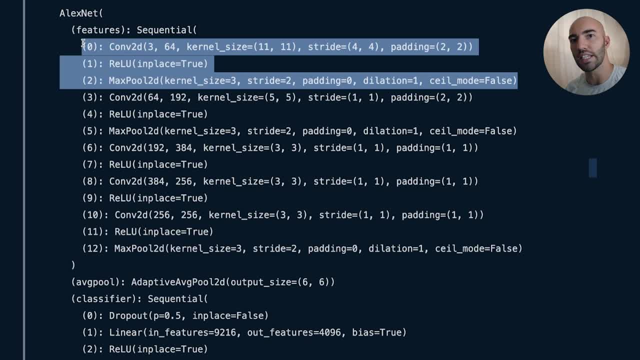 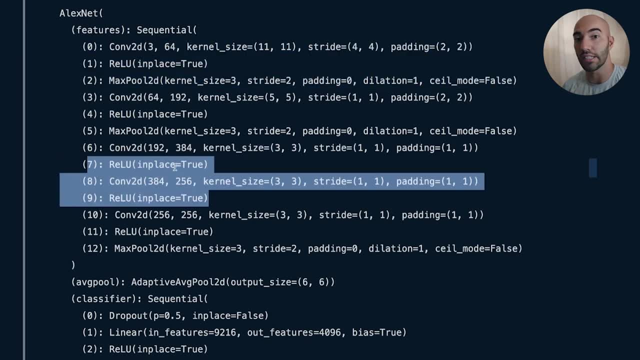 the abstraction sort of feature that's been extracted is like: okay, there's some straight edges here and some curved edges here. We'll go a little further and this is like: okay, this is an animal or this is a fish. And then, by the time we get to here, it's like: okay, 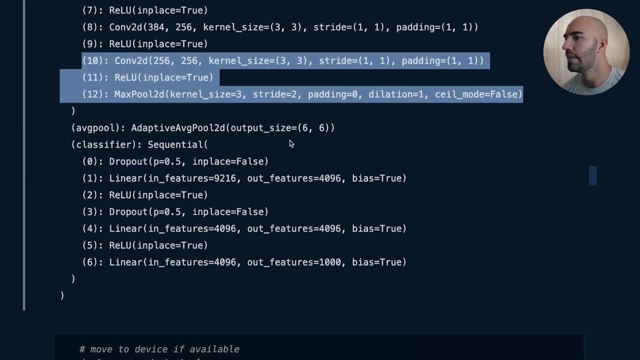 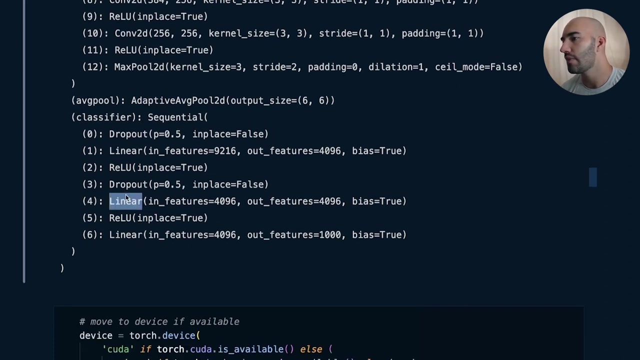 is a goldfish, Hopefully. And then we move on to the classifier part. So the classifier is these three layers. So we have dropout. This dropout was added to reduce the chance of overfitting and improve the ability of the model to generalize. And, yeah, we have these linear, linear, linear. Okay, so these are the 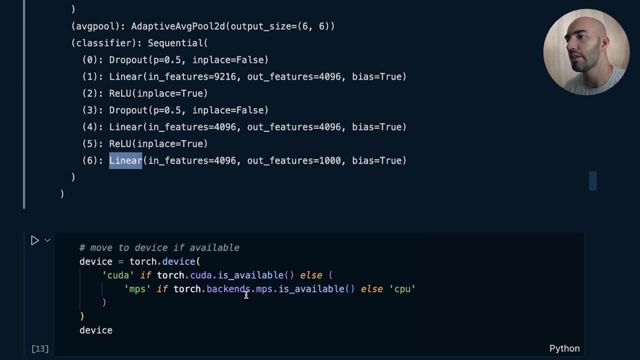 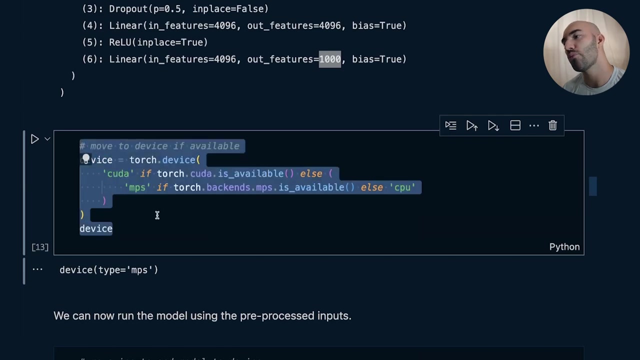 linear layers, The fully connected linear layers that produce the final 1000 activations, And the highest of these activations represents the class that the model is predicting as being that, the class that identifies the image that it saw. So that's the model. We've initialized it. If we can, it's better that. 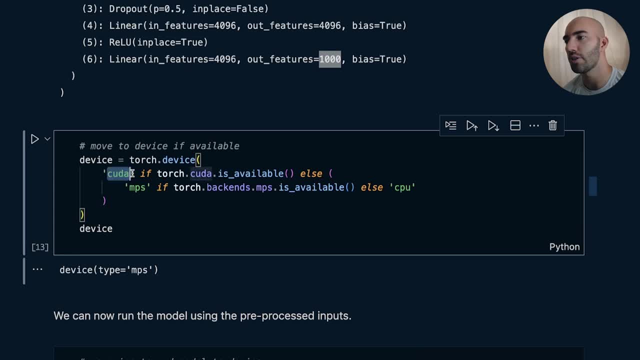 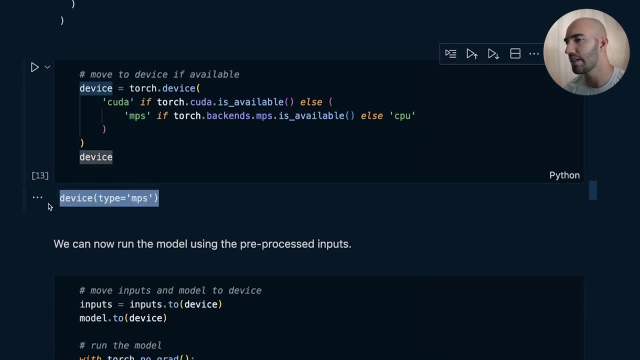 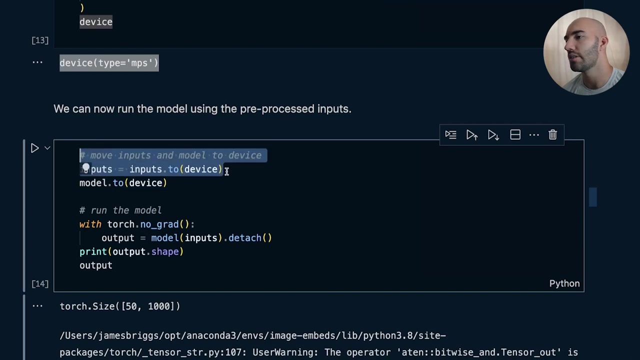 we move the model over to either a CUDA GP, if available, Or, more recently, we have the Apple silicon chips. So if you are on a Mac with Apple silicon, you'll want to use MPS. Okay, so that's the case for me. I have a. I'm going to run all this on MPS. So we move the inputs to the device and 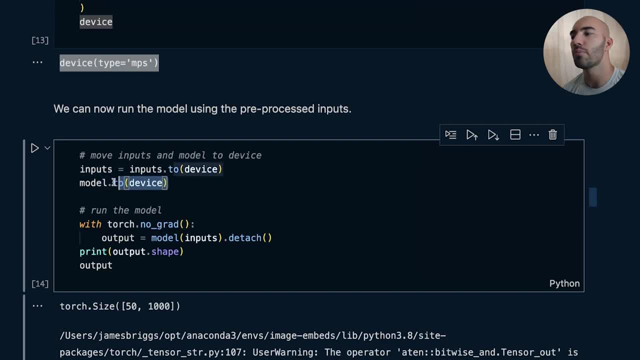 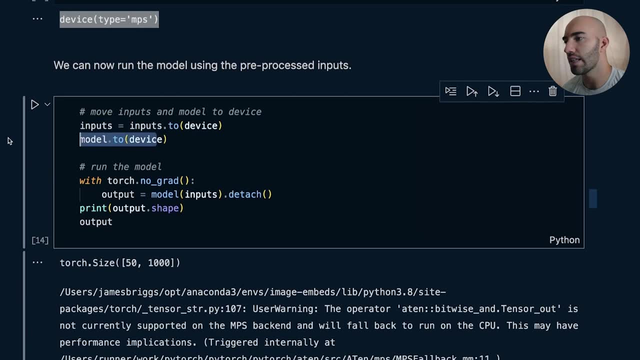 we move the model to the device. Now, when we move the model to the device, it does this in place, so we don't need to, like we did here where it's inputs equals. We just write this And then we run the model. So we set torch, no grads, so we 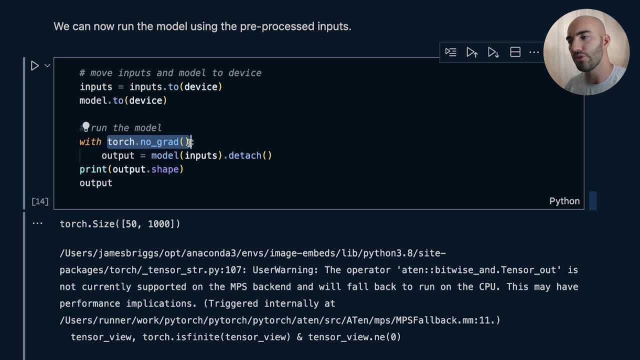 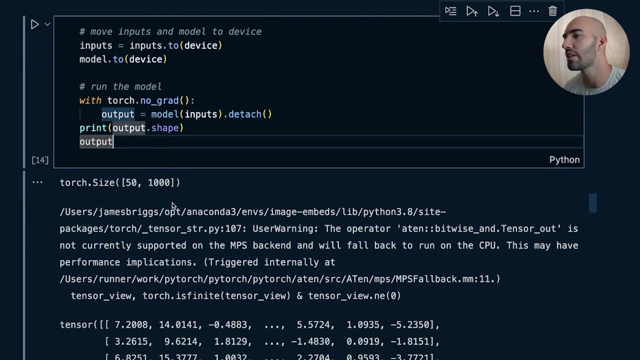 don't need to calculate the gradients, because we do that for training the model. We're just forming inference. So we get our outputs, We detach them from the model and then we can see the shape. So we have these 50 vectors of 1000. 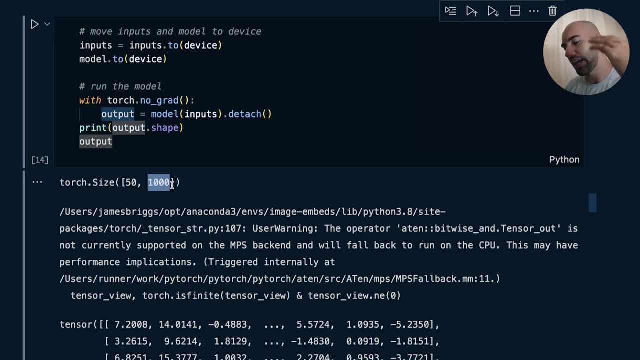 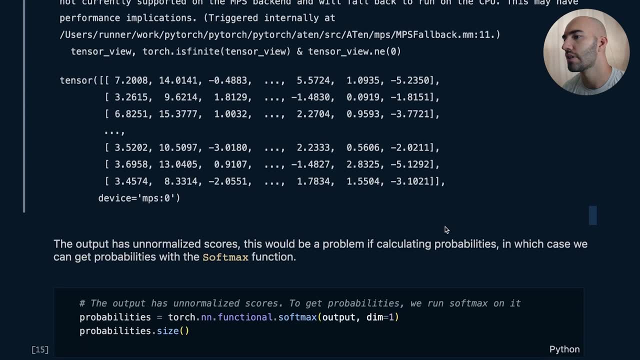 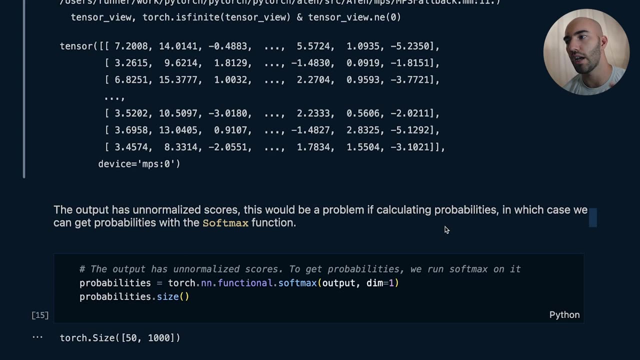 items. So that's 50 activations across all of our 1000 classes And we can see those here. OK, Now these are not normalized. So if we, if you want to calculate the probability from this, we use the softmax function. So we would do. 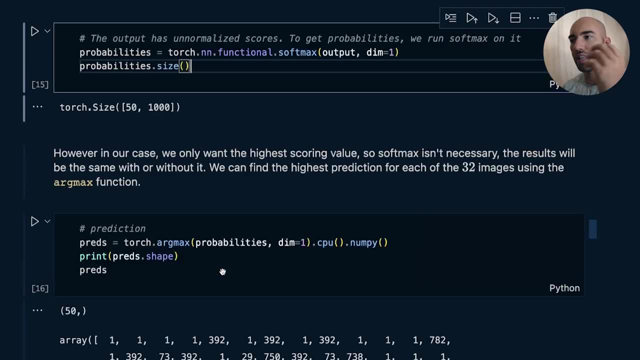 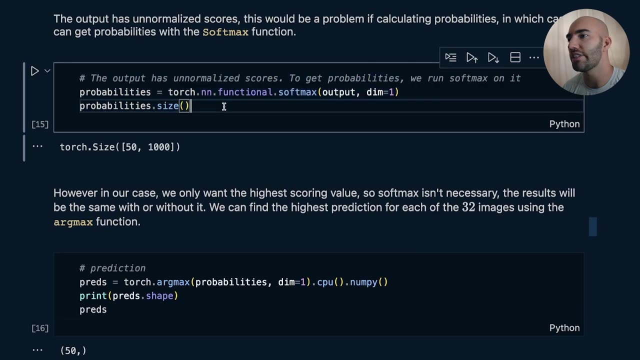 that like this: OK, That that would map everything to a probability distribution and you'll be able to get a probability of, might say, the top five classes, for example. But we don't. we don't necessarily need to do that For what we're doing here, so we could actually skip this. So up here we are getting the 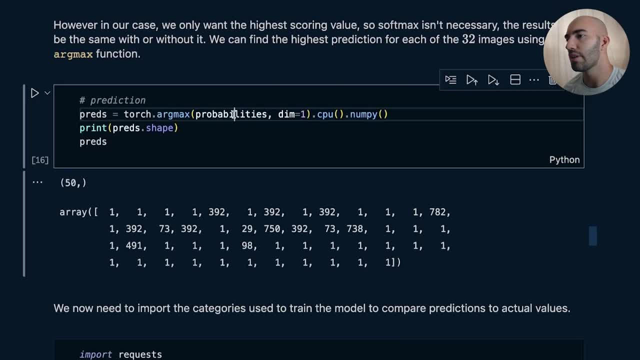 output. So we could skip this, the probability part, and just replace our output, and we will get the same result for what we're doing here, which is taking the value or the index position of the maximum value out of those 1000 classes. So here we're getting one. 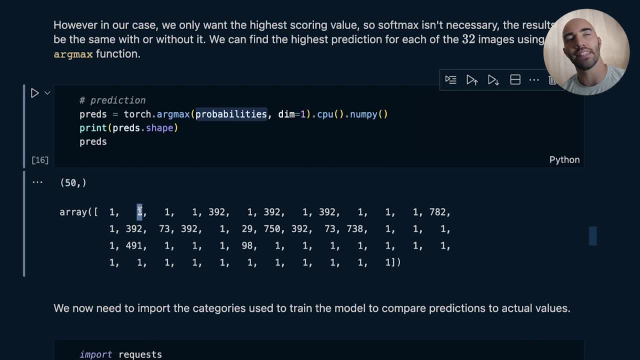 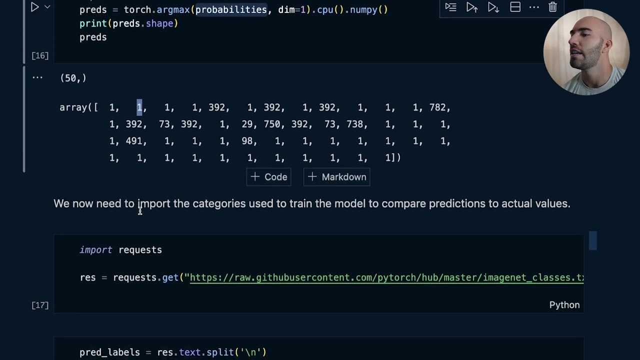 OK, Now, if you remember earlier on, the labels that we had in this data set was zero for the, for the goldfish, And the reason these are different is because the data set actually uses a different set of labels. So it's it's not actually the same, But if we, if we do this, 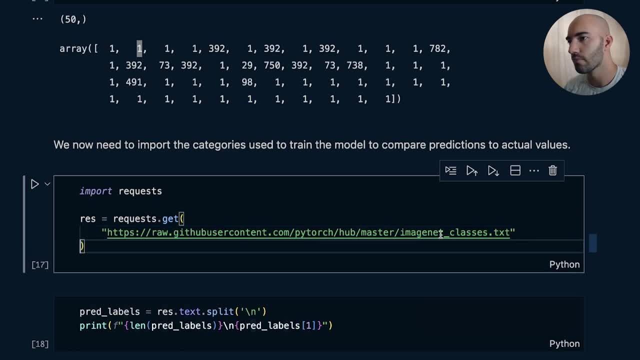 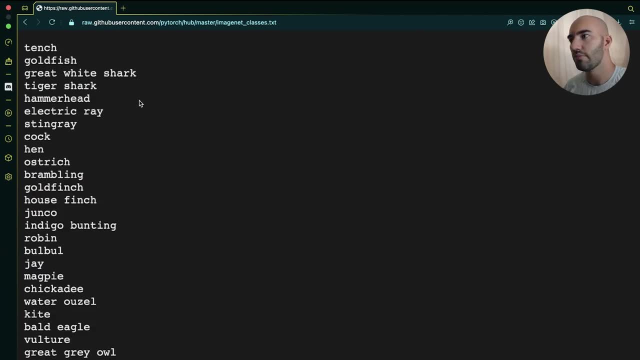 So over here, let me open this and show you. So over here we have a text file where each class is separated by a new line character. So this is number zero And number one is a goldfish Right. So if we get that information, So number one, we can see. 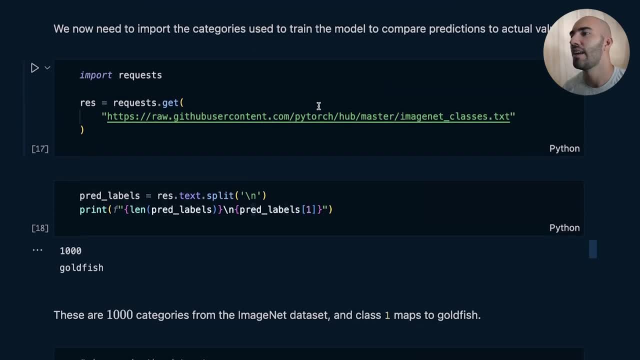 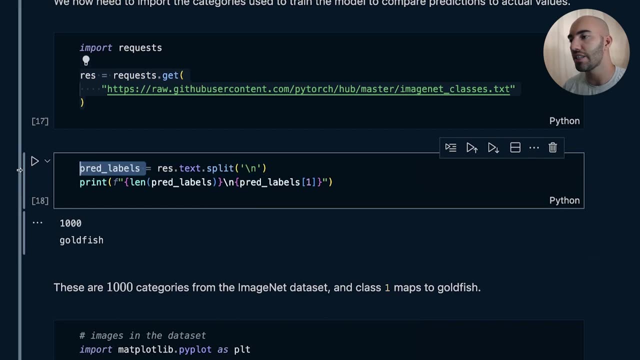 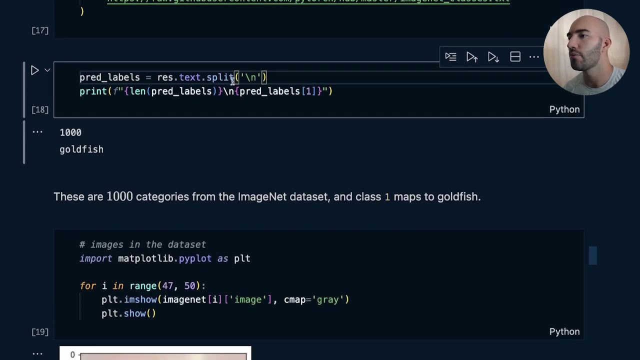 there's a lot of goldfish predictions here, which is a good sign. We can import those, those classes, and we can create a spread prediction labels by just splitting the response we get from this by new line characters. And then what we do is: if you print out prediction 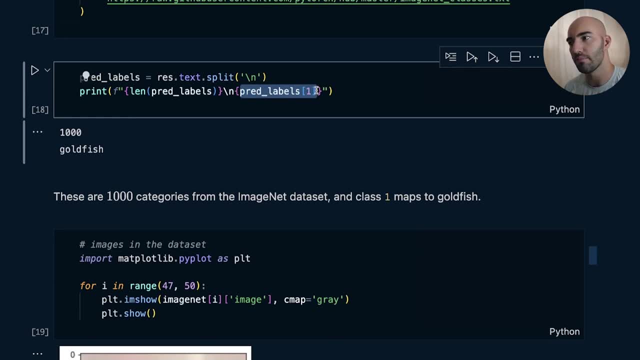 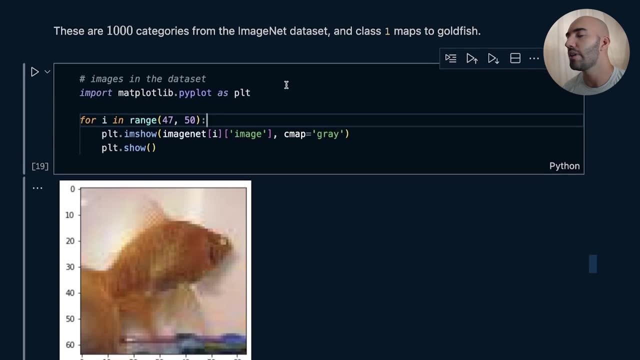 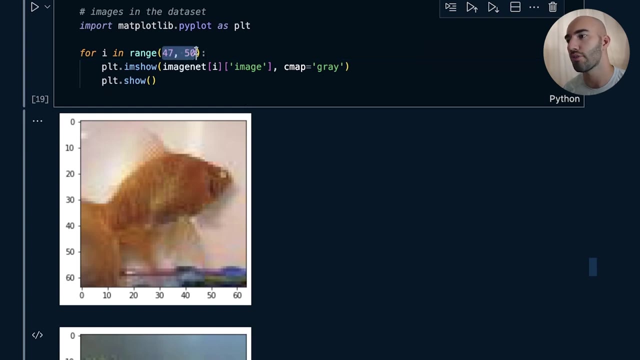 labels. Number one: we get goldfish. OK, So the text label for that prediction. And yes, so we have the first 50 images. All of those are goldfish and we can, we can see here. So I'm just printing out last three. See, they're all goldfish, So we would expect everything all. 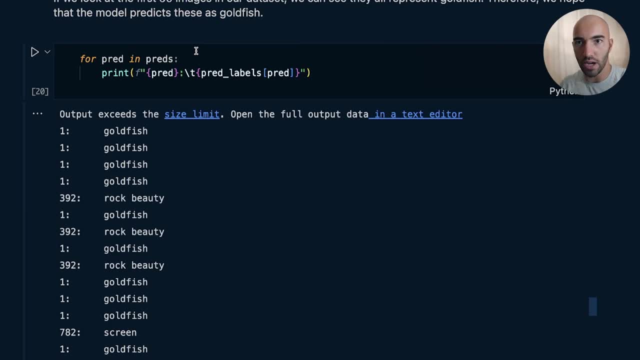 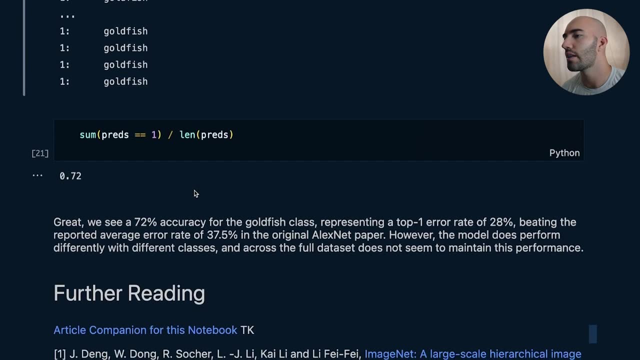 of these predictions to be goldfish. if the model is performing well, OK, And yeah, we see for the. for the most part, that is the case Right Now. if we calculate the performance or the accuracy here, we get 72 percent. So that represents. 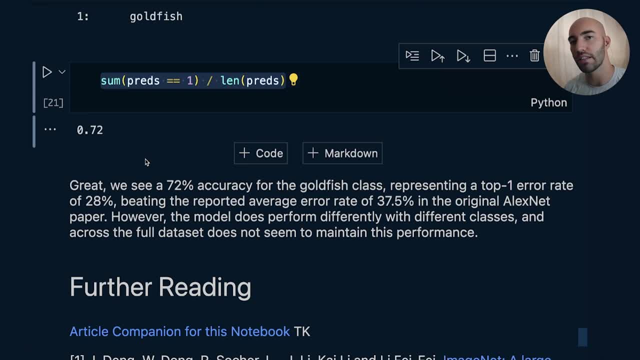 a top one error rate of 28 percent, which beats the reported error rate of the AlexNet model in 2012 on the ImageNet challenge, which was 37.5 for the top one. However, this is. I will point out that this is just a single class. 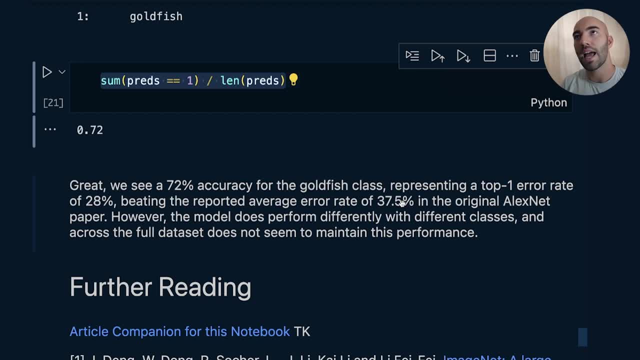 this is a single label, goldfish, right, and the model will perform better on goldfish than other things. okay, so when we test this across the, if we test this across the whole data set one, we have to map all of the different labels between the, between the alexnet model and the data set that. 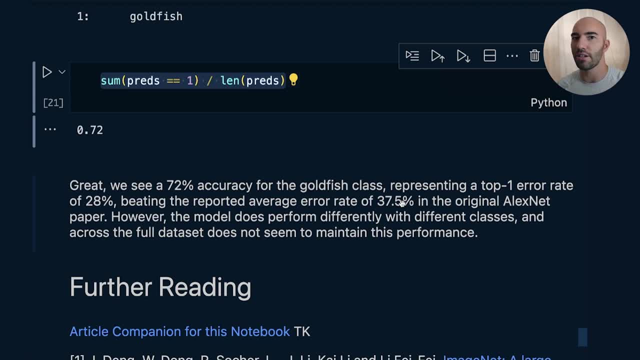 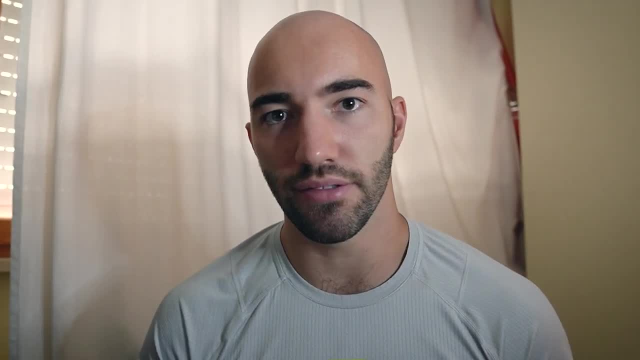 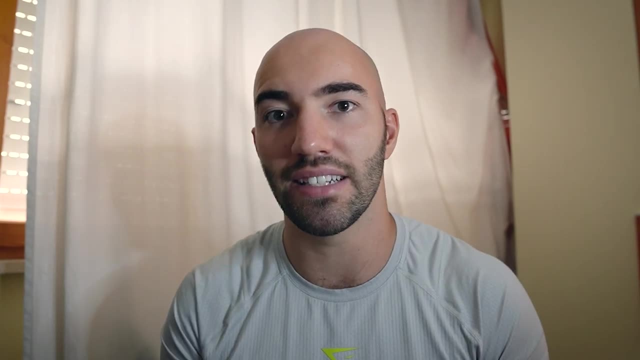 we have here, because the labels have kind of messed up so takes a bit of actual work, but if we do that, the performance will not be as good. nonetheless, i think that is a pretty good result. so that's it for this video. that's our overview of one of the most significant events in computer. 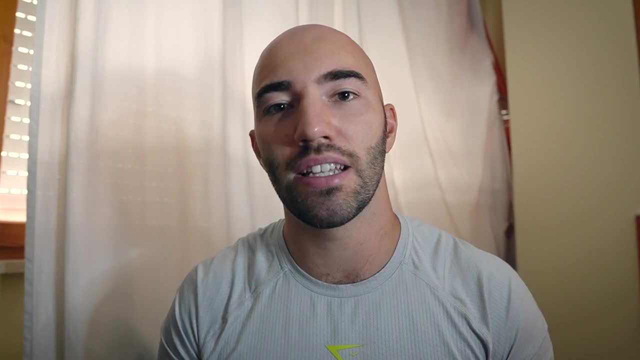 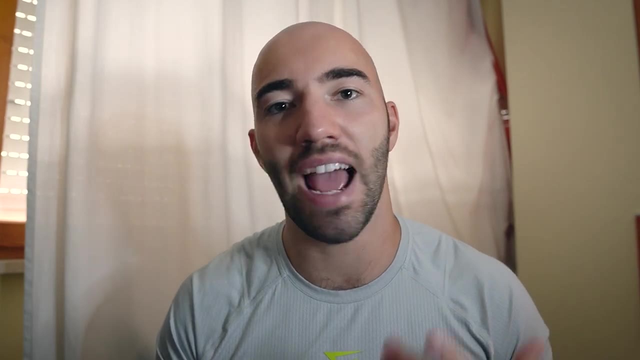 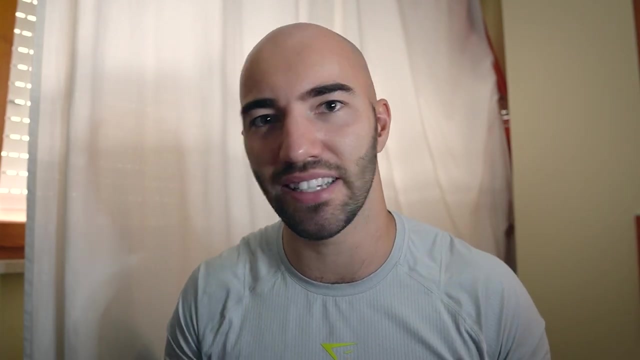 vision and deep learning. the image net challenge was hosted annually until 2017. by then, 29 38 contestants had an error rate of less than five percent. so they're you know, over those years the model was the progress in computer vision just kind of went crazy. alexnet ended up being superseded by 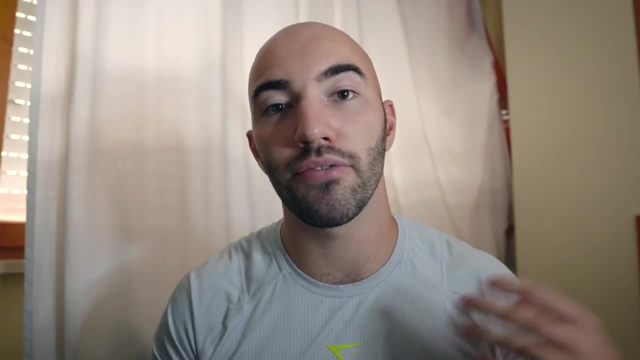 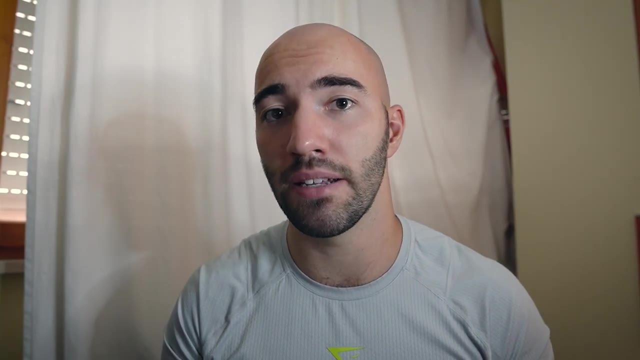 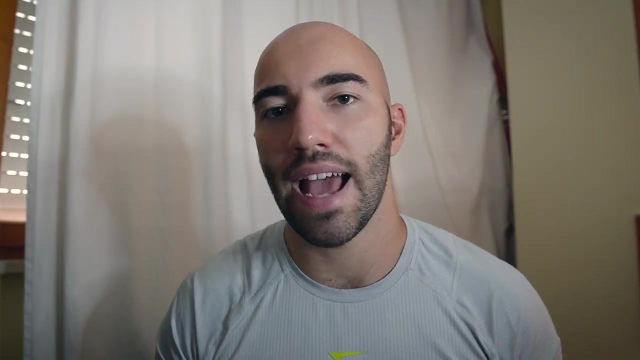 even more powerful convolutional neural networks. microsoft research asia was the first other team to beat alexnet, and they did that in 2015, and since then there have been many other sort of state-of-the-art convolutional networks that have come and gone, and even more recently there are the 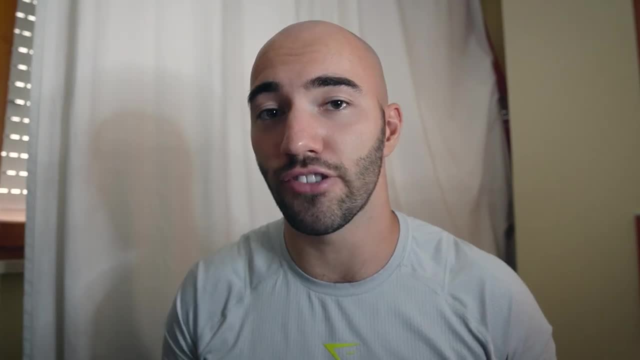 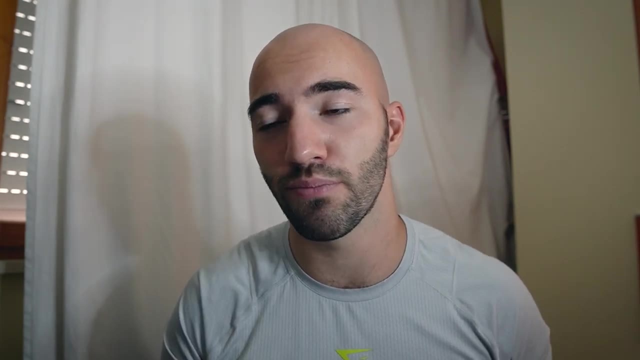 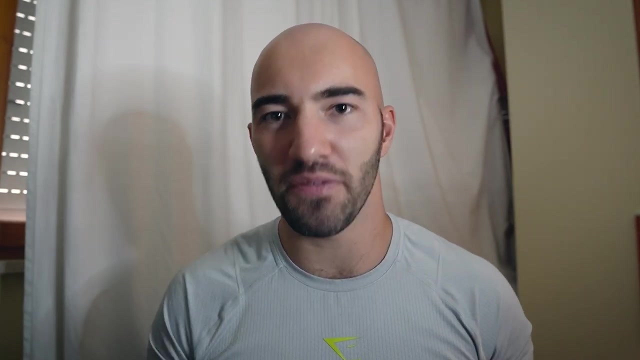 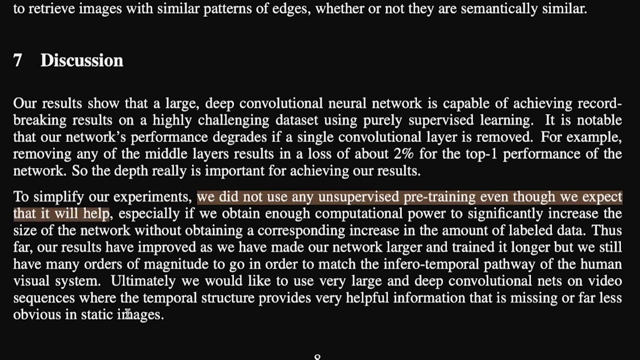 possibility, other networks coming in, such as transform harmonics and disrupting the dominance of convolution neural networks in computer vision. now i'll leave you with the final paragraph of the the alexnet paper, because it's almost seems like they saw the future of deep learning. they noted that they did not use any unsupervised pre-training, even though they